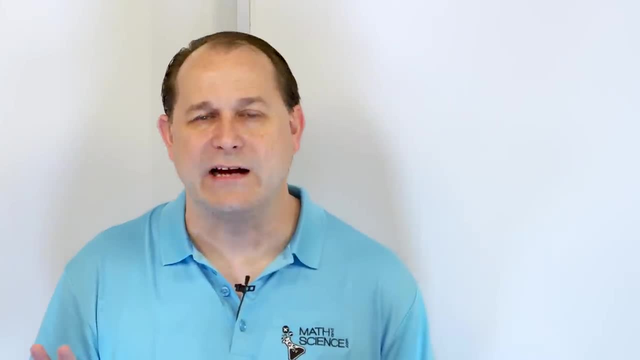 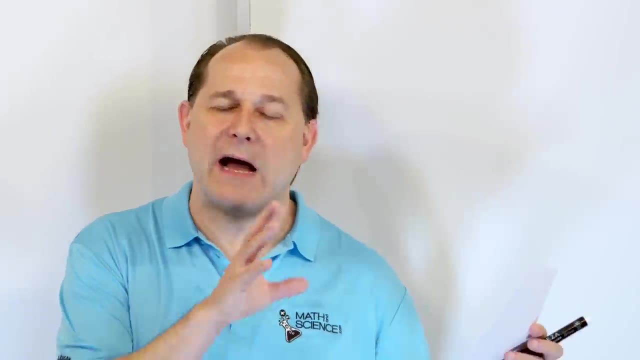 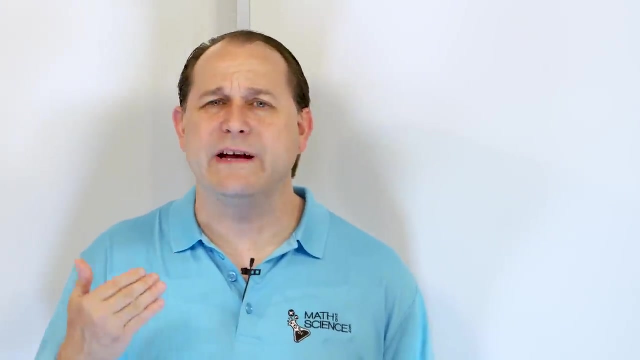 a historical treatment of how the discovery of the electron really happened. because, number one, it's fascinating. Number two, it can give us some clues into the thinking behind chemical concepts that we need to consider going forward. And the other part of it is in this class. I really want to introduce, as best I can, our modern 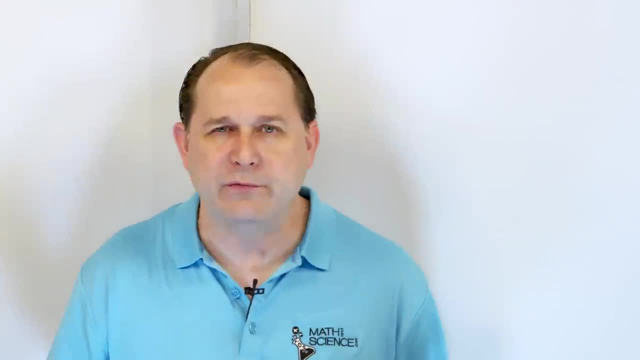 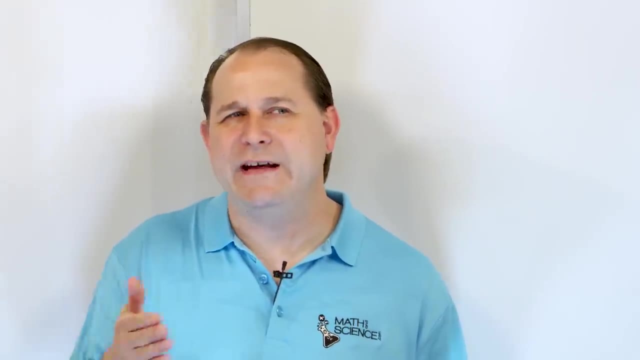 thinking about what electrons really are and also what photons really are, which is light waves? right, Because as we get farther and farther into chemistry, you start realizing that your teachers have been lying to you as you learn early chemistry in most books, in most classes. 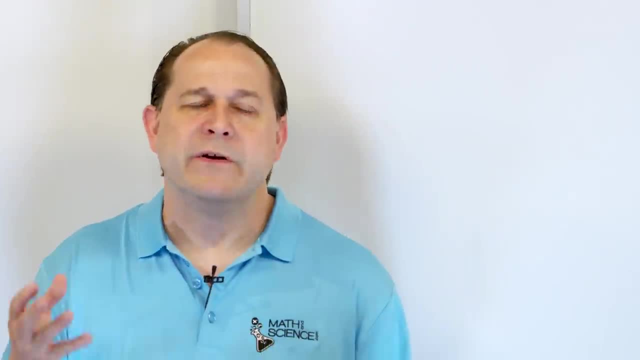 I'm going to try to lie to you as you learn early chemistry in most books, in most classes. I'm going to try to lie to you as little as possible. So in the beginning we have a model of the atom, which we're going to talk about more later, where you have the protons and the neutrons. 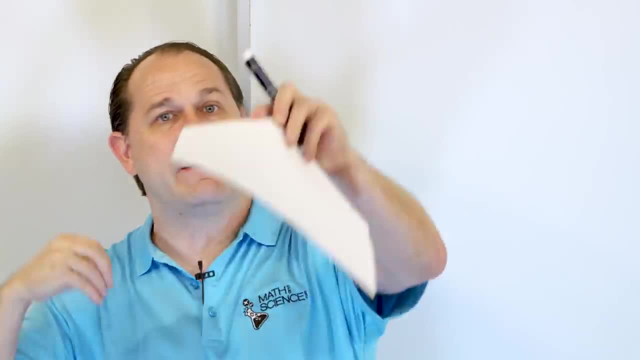 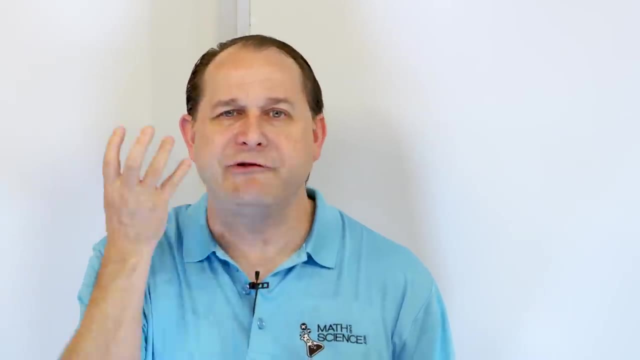 in the center and you have the electrons which are surrounding and we think of them as orbiting like solar system, like planets in the solar system. That's a very useful picture to have in your mind And, of course, it is the model that the early pioneers had also. That's what 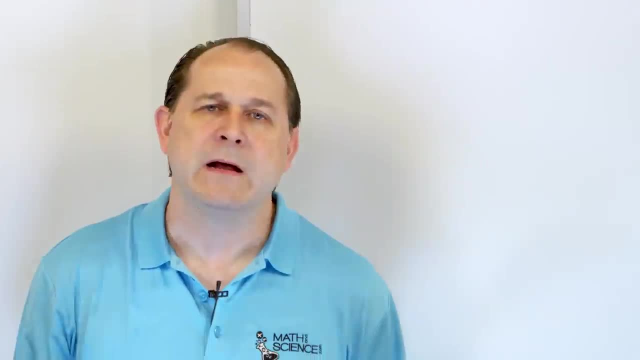 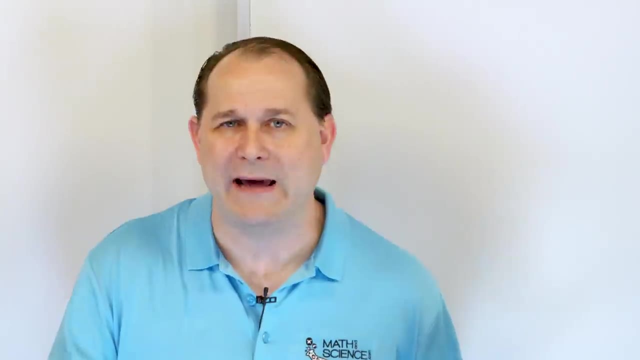 they thought it was was electrons orbiting like planets around the sun. right, But as we get farther and farther into chemistry, you start realizing that the electrons are not and do not behave like planets going around a solar system, And all of our modern usage of 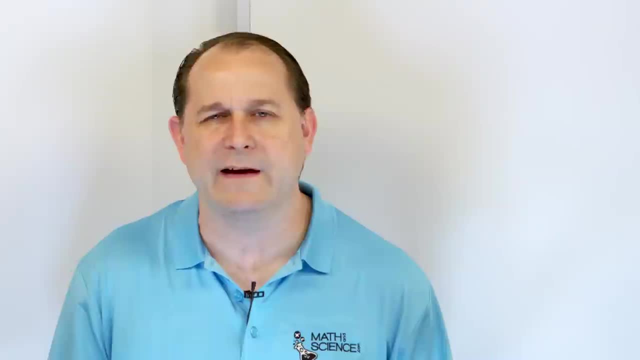 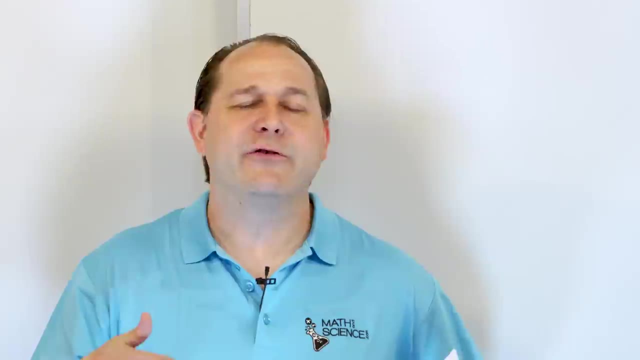 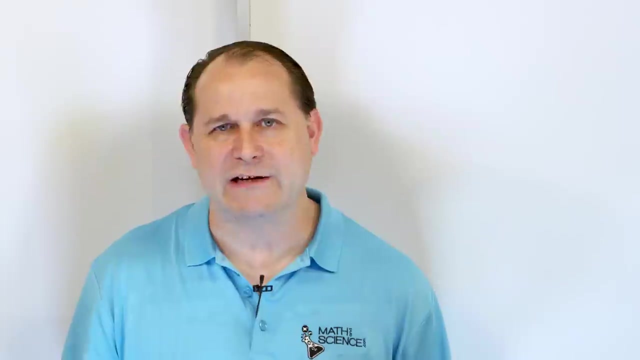 chemistry- organic chemistry, synthesizing drugs and other things- is absolutely dependent on our understanding what electrons are, because electrons govern chemistry right, And so if we can better understand what the electron is, then of course we can apply that to developing modern technology. 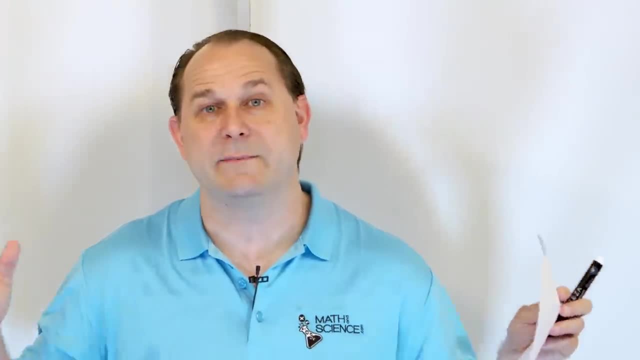 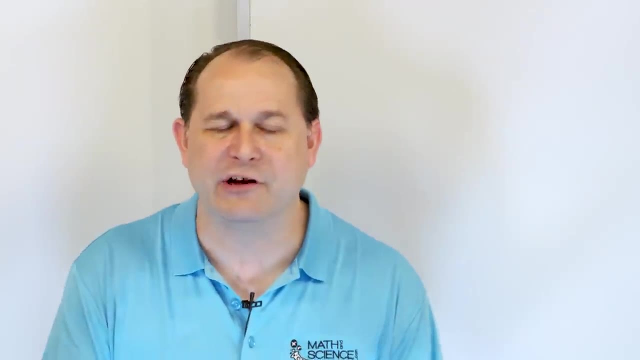 Now the whole concept in field called quantum mechanics is basically talking about what is an electron? how does it behave? There's something called a wave function. We're going to talk about that kind of stuff much, much, much later Here in this lesson. we're just going to go back in time. 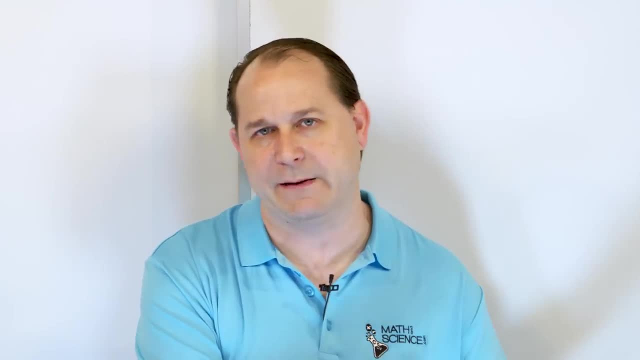 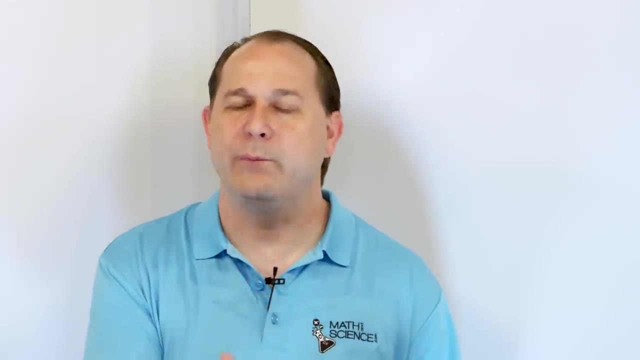 before we knew anything about quantum mechanics, before we knew anything about quantum chemistry, before we even really knew the structure of the atom at all, and talk about how the electron was discovered and what we learned about that, And then in the next lesson we'll talk about 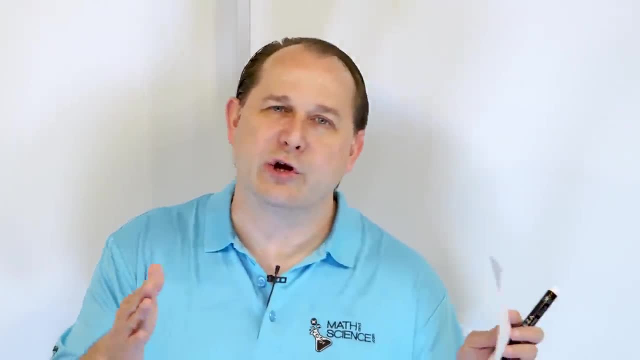 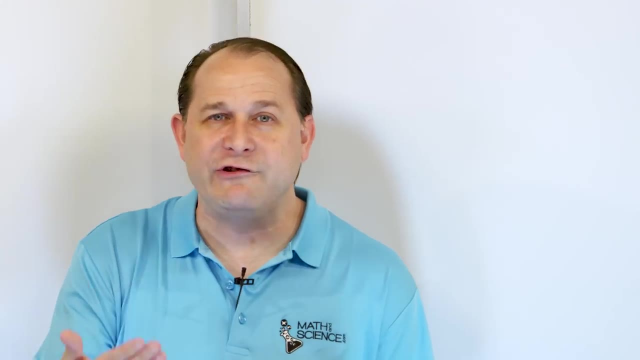 remaining parts of the atom, the neutron and the proton, And then, as we learn, the chemical concepts beyond this point, knowing that these ideas were discovered in this way, we're gonna modify them and change them with our current understanding. So in a few chapters down the road, 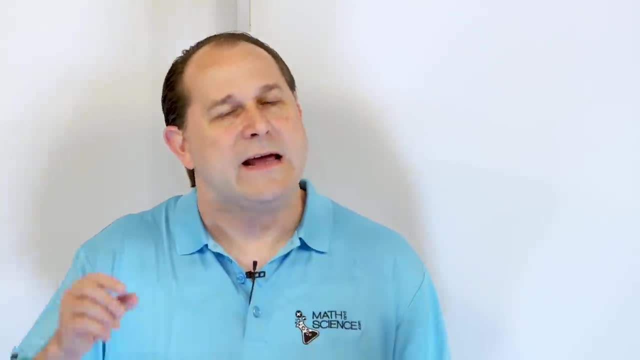 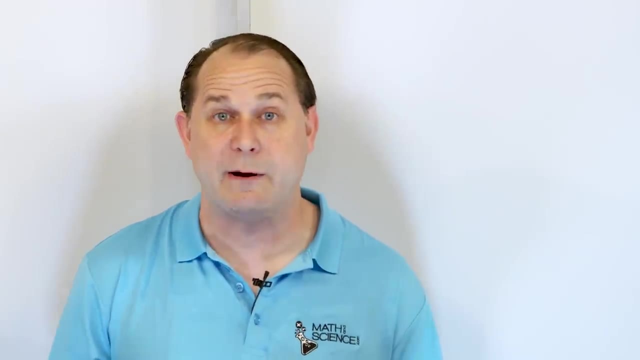 you'll understand exactly what we actually think an electron is, And I'll give you a spoiler alert. It is not a little ball that goes around the atom. It does not behave like that with our current experiments and knowledge that we have about how electrons 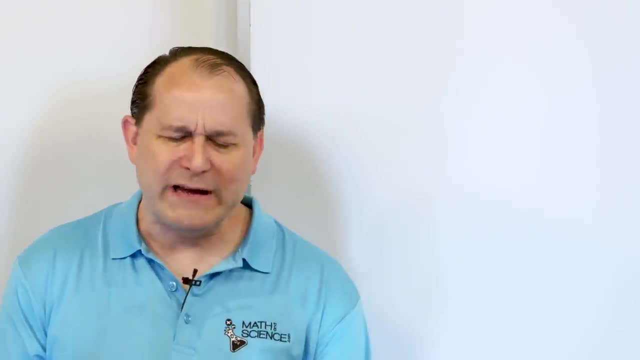 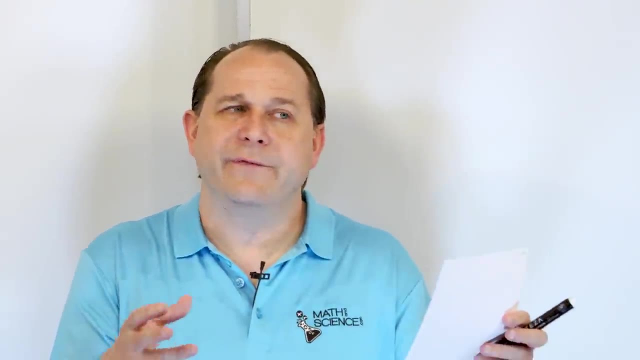 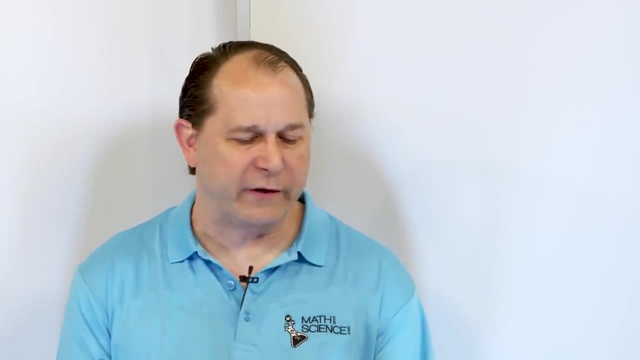 and protons really behave All right. So in the early or the late 1800s experiments were done with atoms to try to figure out what they were composed of, And one of the earliest experiments that really led to the discovery of the electron 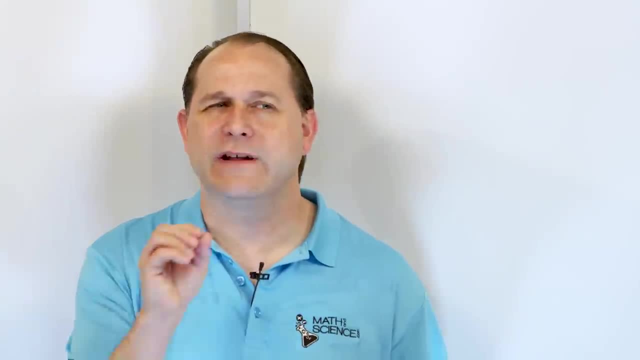 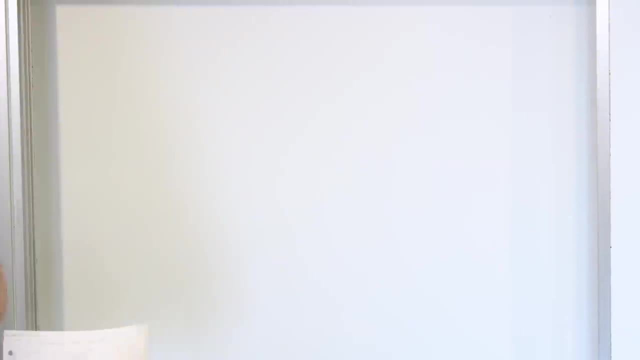 was called the cathode ray tube. You may have heard cathode ray tube. You may have heard the letter CRT. Maybe you haven't. It's okay if you haven't. But basically the idea goes like this: What you do is you take a glass tube. 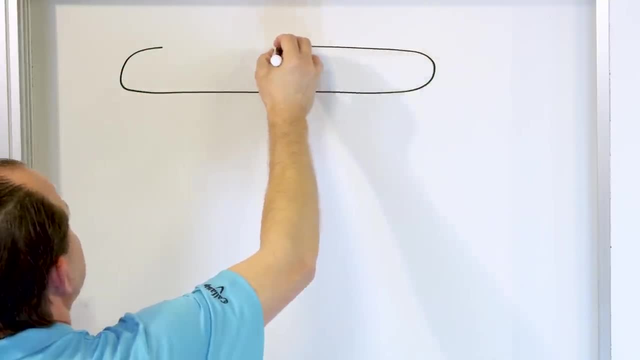 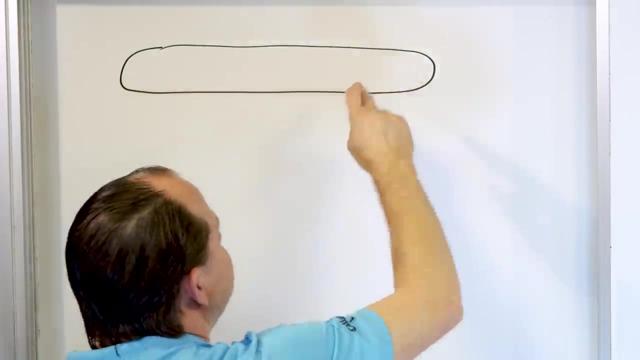 or you know you can use glass. you can use quartz, which is another clear, glass-like looking material, And what you do is you pump out the air and make it a partial vacuum in here. You don't want too many atoms inside of it. 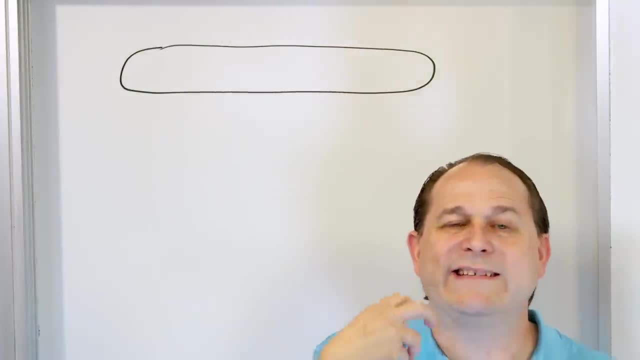 because what you wanna do is you wanna excite the gas with electricity, And the more atoms are in there, the more energy you need to excite all the atoms in there. So what you do is you pump out a good chunk of the atoms that are there. 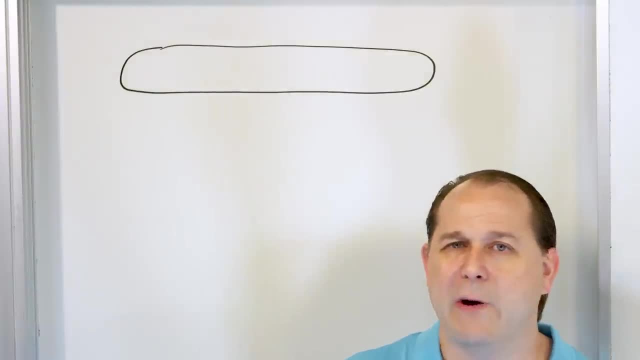 Maybe you even fill the tube with a different gas than air, because you know air is nitrogen, it's oxygen, and there's other trace gases as well. There's carbon dioxide in the air, and so on. You may have seen the neon tubes. 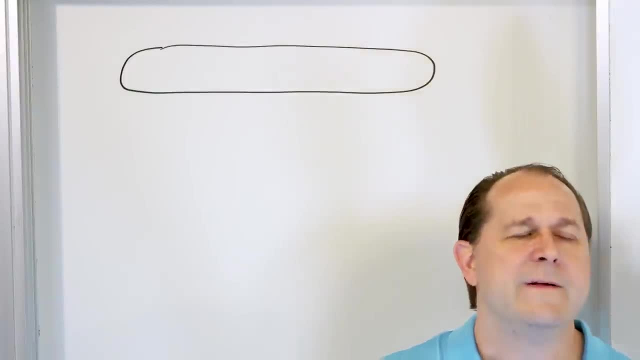 which glow a certain color. right, The orangish, reddish glow. You could put a tube full of neon gas or argon gas. We can make different colors by putting different gases, But in the earliest experiments we didn't put any special gases in there. 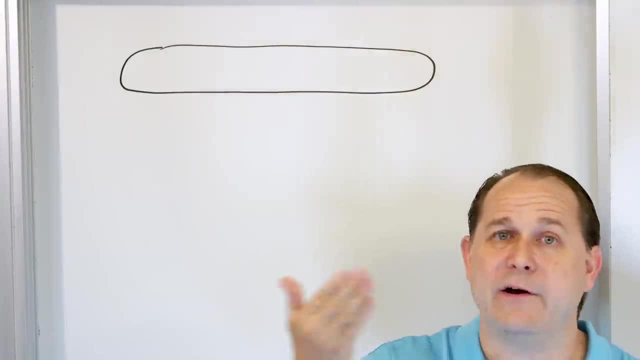 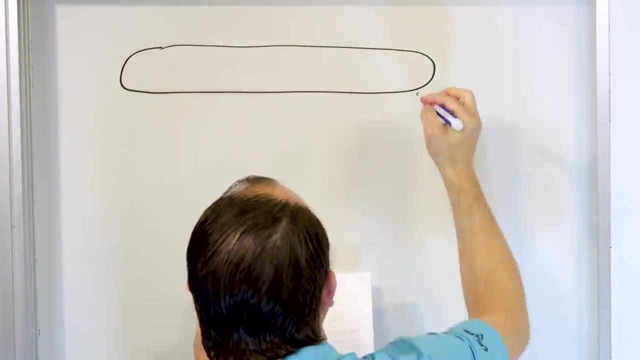 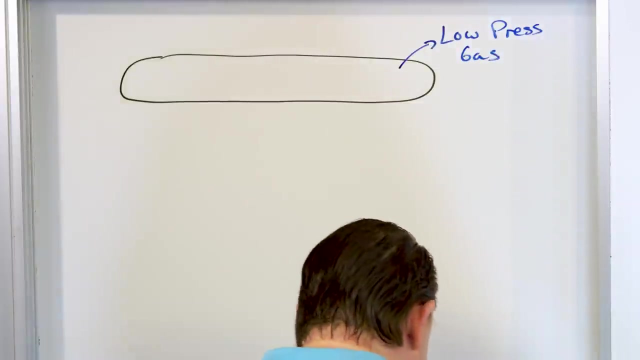 We just pumped out the atmospheric gases and just made it a low pressure tube there on the inside, All right, And this side of this really is a gas, but it's a low pressure gas. So low pressure gas, All right. And then what you do is you hook up to that. 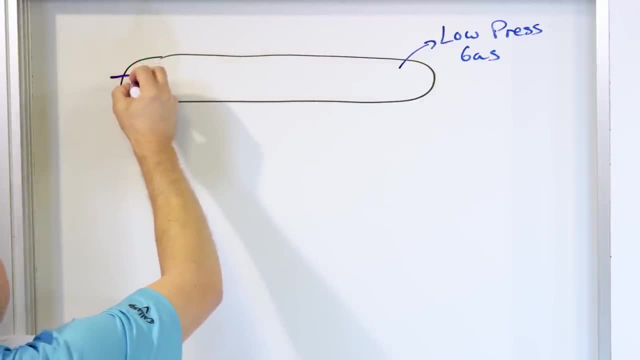 You put a metal terminal which kind of penetrates the glass but it's still sealed So no air can leak out right. So it kind of penetrates that right there And it's a metal piece of metal there And you do the same thing on the other side. 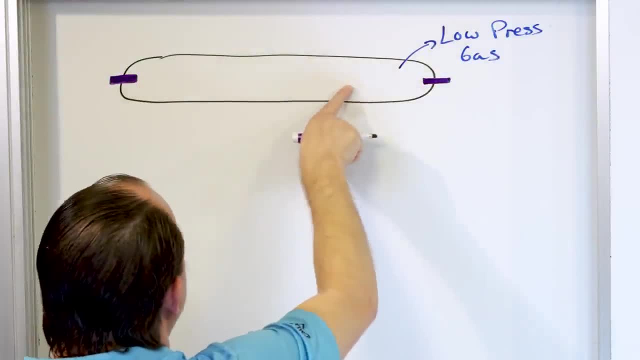 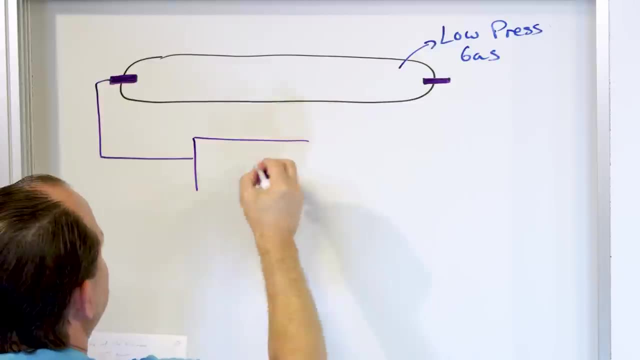 You penetrate the other side So it goes through, but it's still sealed and no air can really leak out. Right, So it's still sealed and no air can leak out, leak out of this area right here. And what you do is you hook this guy up to a high voltage source. 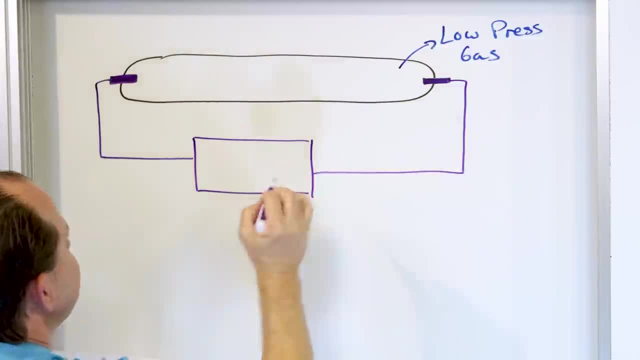 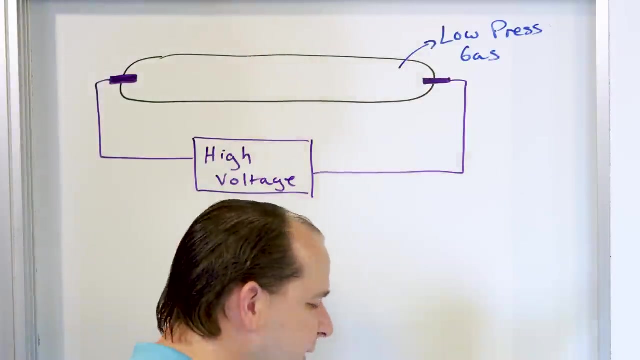 Now I'm not going to go into the details of exactly how they generated the high voltage source, or if it was alternating current or direct current or how much or whatever. All we want to say is that this was high voltage And what we do then. when you have a voltage source, you always have. 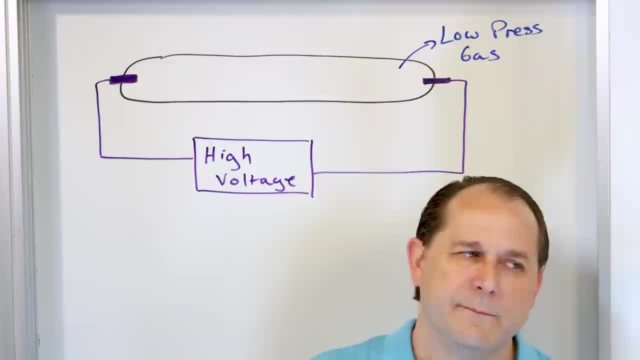 a positive terminal and a negative terminal. Now we know- back in the day we didn't know this, but now we know- that electricity is the movement or the flow of electrons in the circuit. Electrons are in the outer shells of all of the atoms, and so they can much more easily move freely. 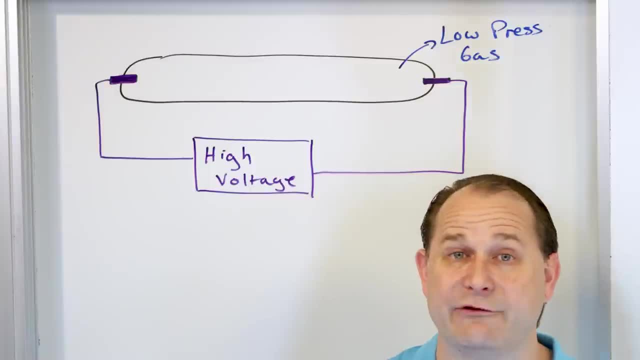 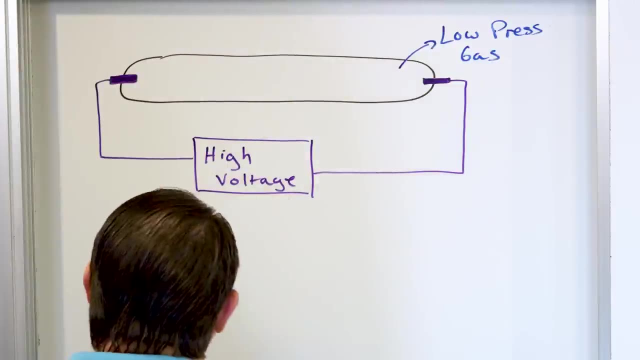 They can bounce between atoms, And so when you excite an electric current, we now know that the electrons are the thing that's moving through the wire. So there's a positive and a negative terminal involved in every circuit, involved in every battery. So in this drawing, this is 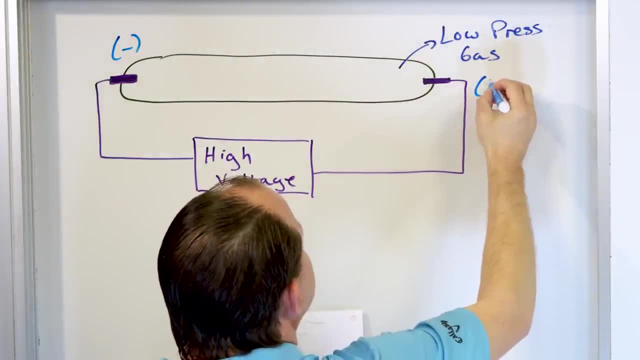 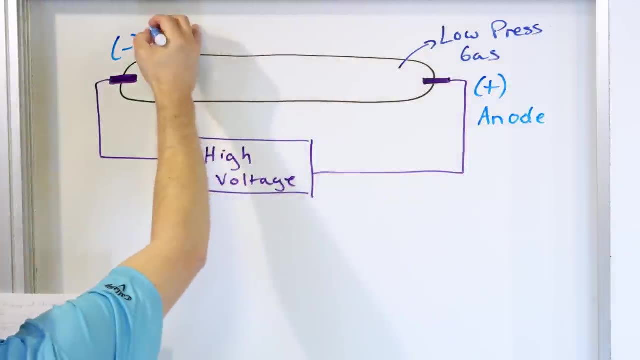 the negative terminal And over here in this drawing, this is the positive terminal. Now, the positive terminal we call the anode And the negative terminal we call the cathode. But I want to caution you not to get too hung up with the words anode and cathode. 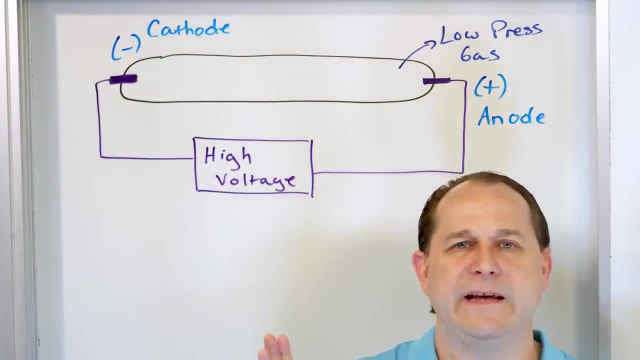 because I'm going to tell you right now, it's very confusing Because the definitions for anode and cathode can kind of change depending on what you're doing. If you're charging a battery versus discharging a battery, are you talking about electrically? Are you talking about 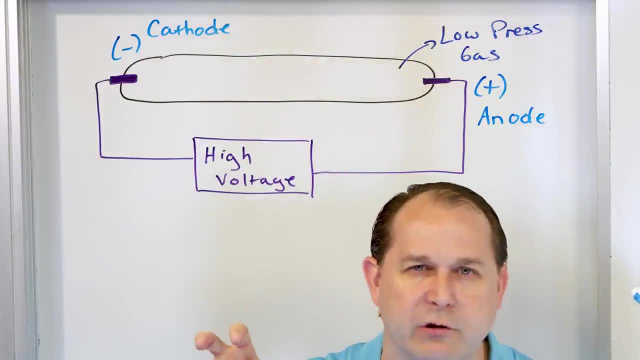 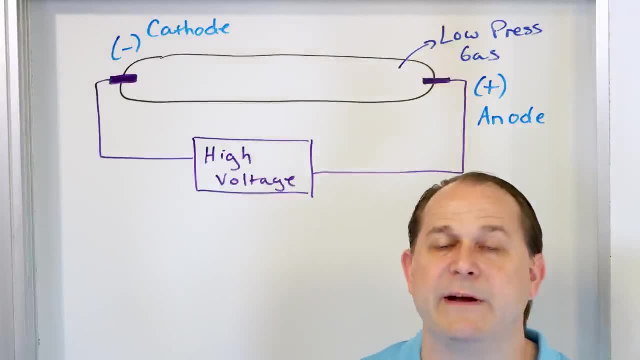 anode and cathode. they might not be the same depending on what you're doing, So I've labeled them in this diagram, But really all I want you to know is that this is the negative terminal, This is where the electrons come out, And here is the positive terminal, which is opposite to the 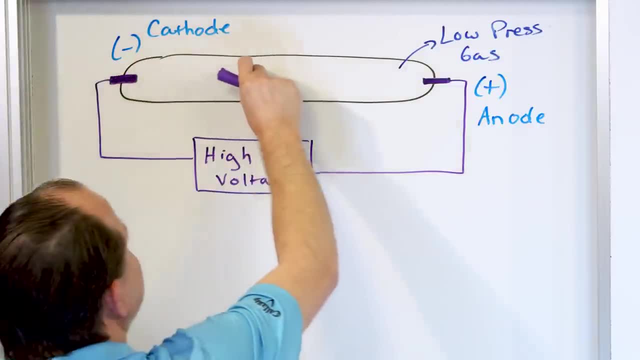 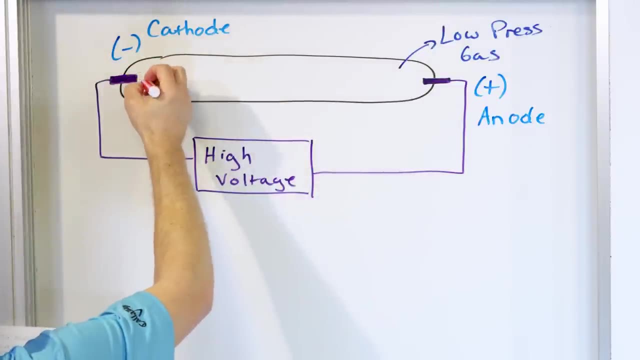 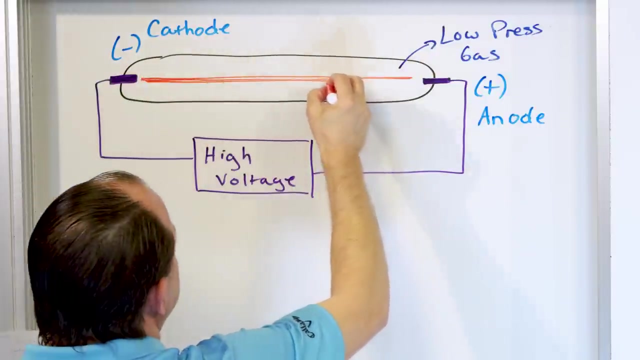 negative terminal. Now, what happens whenever you have a low pressure gas in here and you put a very high voltage across this is that you start to see a kind of like, kind of like this, this wispy ghost like looking discharge. that's happening And it just kind of lights up the interior of this. 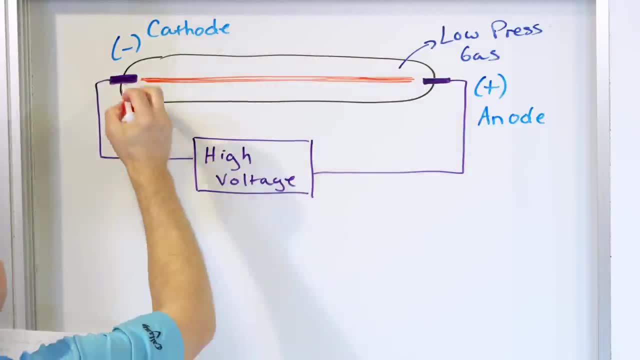 tube. So we now know what's actually happening is the metal here is basically exciting. the gas here, and it's releasing electrons from the, the material that's inside of this, and then they're being accelerated through the gas And then it's releasing electrons from the material that's. 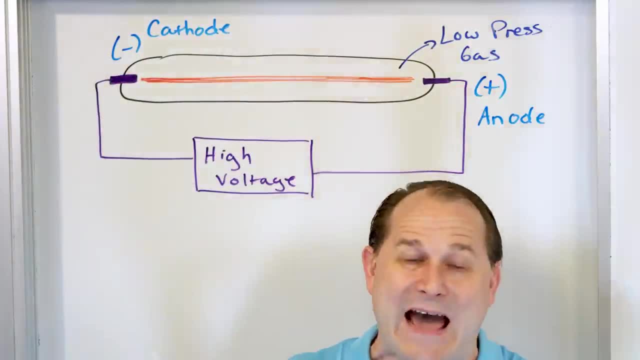 inside of the gas, which also glows, because we now know the gas has electrons that are orbiting there, And when you excite the electrons and when the electrons fall back down, that's when things start to glow. In fact, anything you've ever seen glow, even if you put a red hot poker. 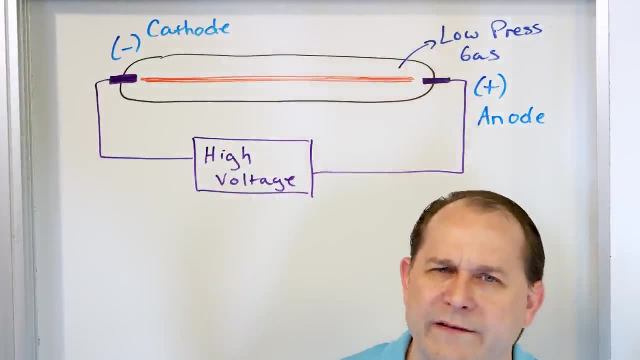 in a fire and you pull it out and it glows. you ever wonder: why does it glow? Like what is causing the light to happen? I mean, did the fire like, store its orange energy and then release the orange? and that doesn't make any sense. That's not what's happening. The fire when you put a. 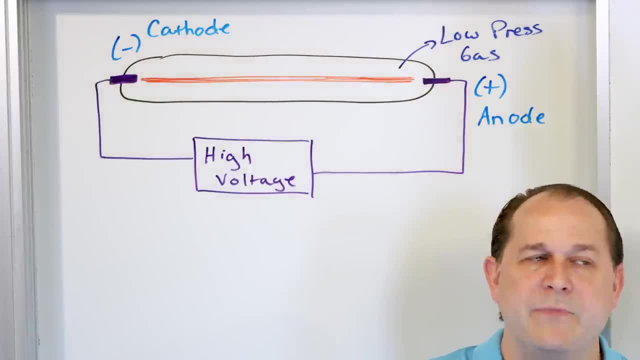 hot poker into a fire. it is heating up the metal And when you release it and pull it from the fire, the metal is still extremely hot and the electrons that are in the outer layers of all of those atoms are bouncing up and down all over the place. because that metal is hot, The electrons are going. 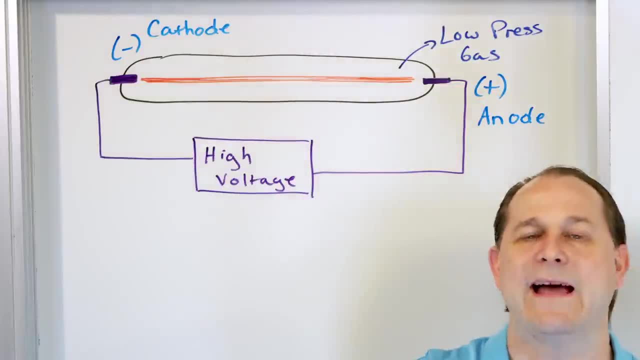 up into a higher energy and when they fall back down into a lower orbit, a lower energy state, they release a photon. Most things that you see that glow like, glow in the dark stickers, things like that. that's all because of. the electrons are falling back into a lower position, closer to the atom. we call that a lower energy. 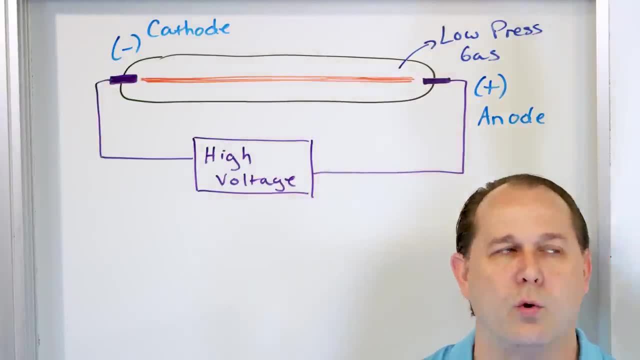 state, and when they do that, when they fall in, they release a photon, or some photons of light which we can see. the red hot poker works like that. glow in the dark stickers work like that, and also this uh, glowing gas works like that too, because the electricity is causing the atoms to pump up and 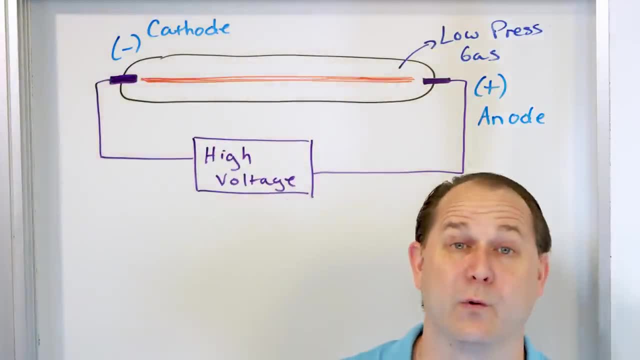 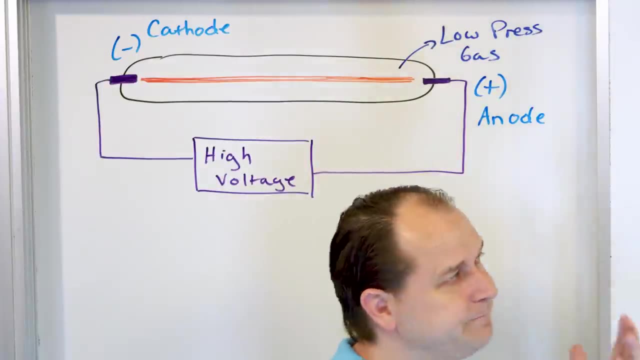 then they come down. when they come down, they release light also. lasers work that way, but we do some tricks to make all the wavelengths line up perfectly and it makes a nice pencil beam. that's what's happening in a laser, but anyway, it was very surprising to see this wispy discharge looking. 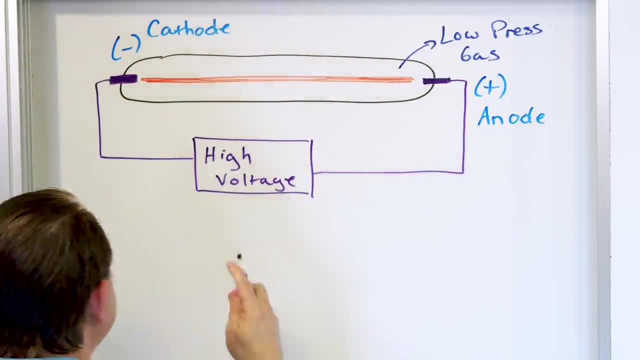 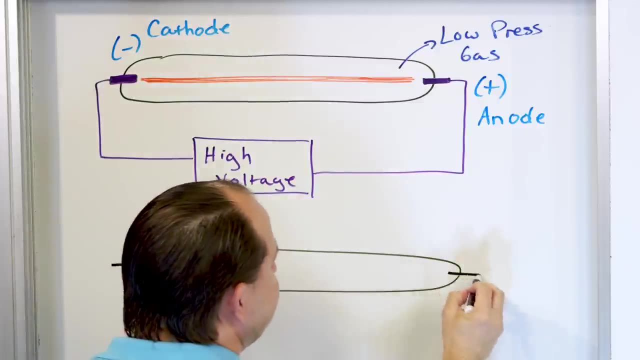 thing: uh here, because what? what? uh the next step here in in that experiment, when we, when they did that experiment, we do the exact same thing. so here's your terminal penetrating in here. here's your terminal penetrating in right here, and, just as before, this is the negative terminal, this is. 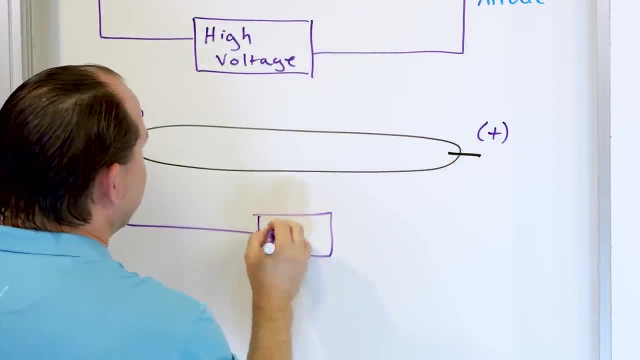 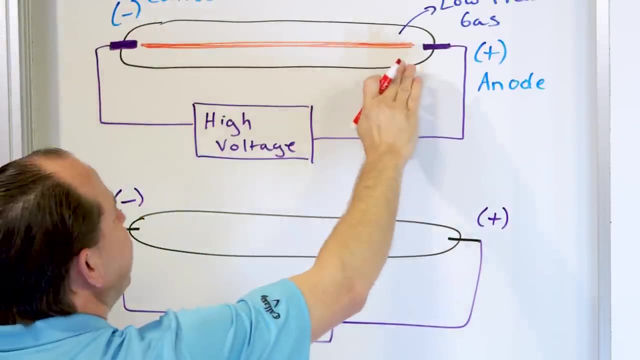 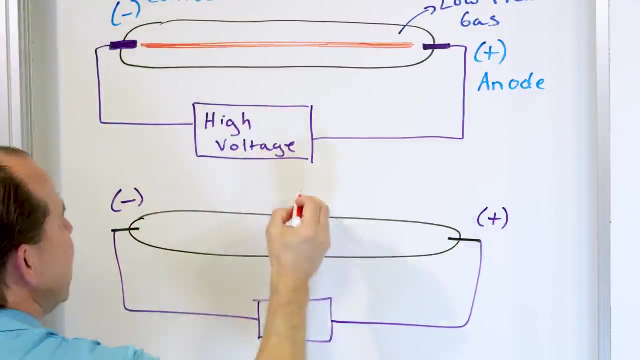 the positive terminal and of course we have a high voltage source. i'll put high voltage source like this right. so what happens actually is if you leave this thing undisturbed, it's a nice straight line going uh directly across to the other terminal, completing the circuit like this right. but actually, if you put a bar magnet, 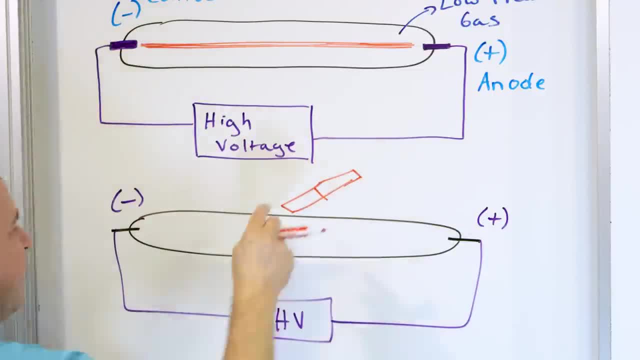 on the outside of the tube, like this right and just kind of hold it close. then what happens is the uh beam of particles. it actually moves. so you can actually take a magnet on the outside of this tube and whereas before it would have continued all the way over. but you can actually. 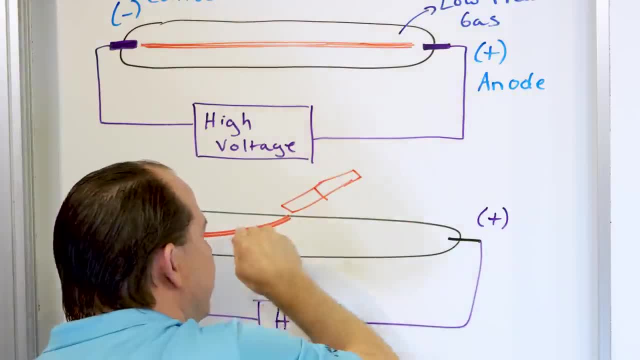 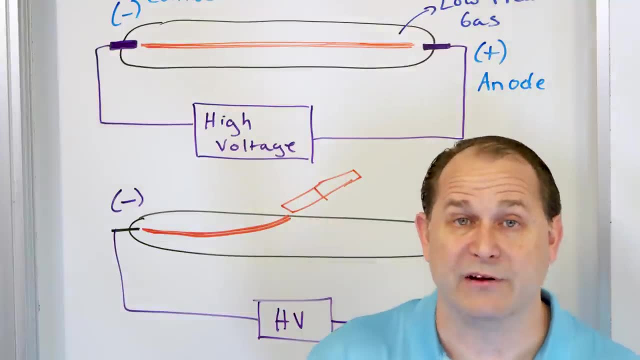 make it impact the glass. you can move it around this way. if you move it over here, maybe it kind of goes farther and then it curves up. basically the beam of these things which the punch line, as we now know it's a beam of electrons. right, it was called a cathode rays. it was called cathode rays. 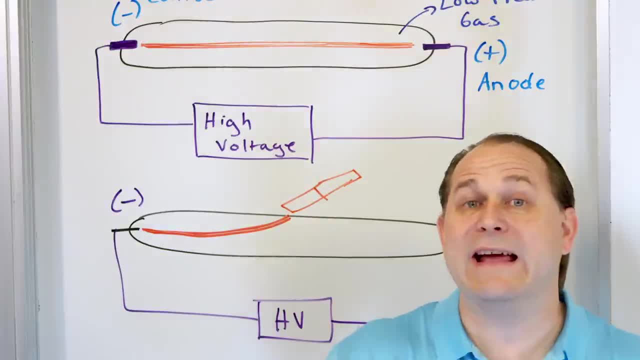 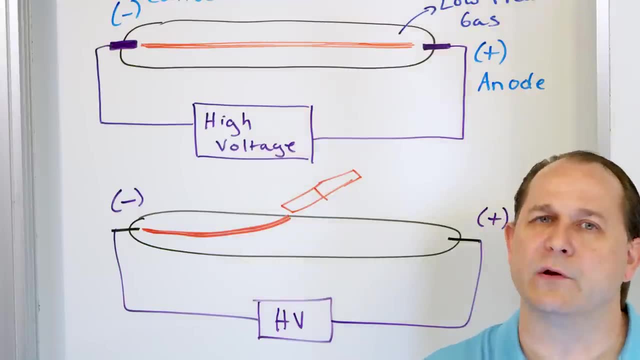 because you have a cathode and you have an anode and these rays appear to emanate from the cathode, so we call them cathode rays. and it's influenced. this beam, this, these rays, are influenced or able to be influenced by magnets on the outside of the tube and also. 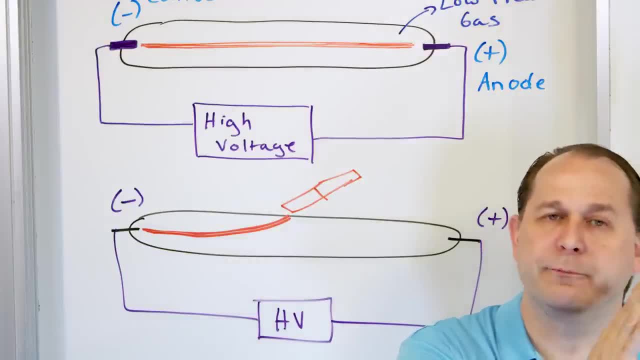 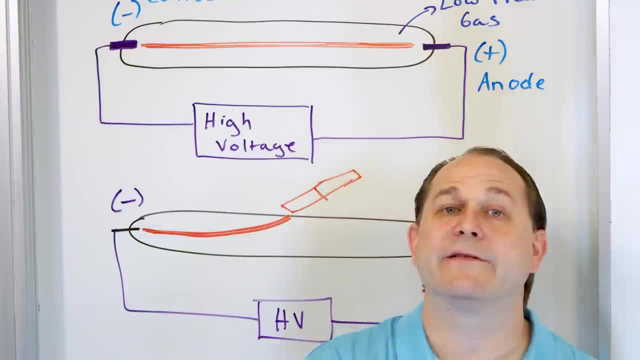 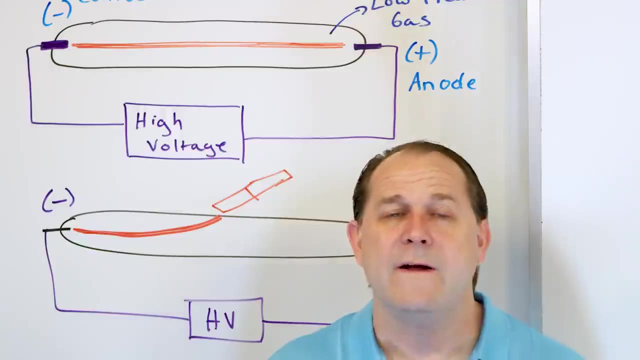 they later learned they are influenced by charged plates, charged electrical plates. so around a magnet is called a magnetic field, around a charged plate is called an electric field. so basically the beam of electrons can be moved around by either an electric field or a magnetic field. so obviously that beam of cathode rays must be a beam of some sort of charged particle. 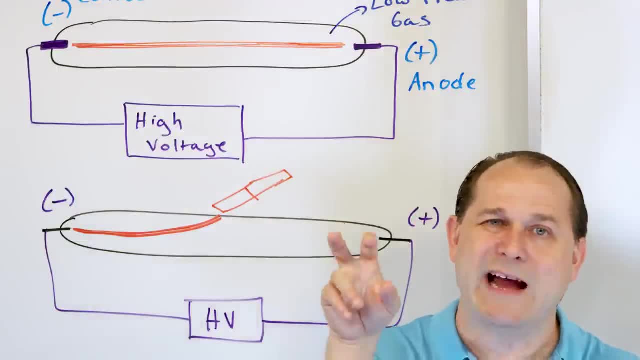 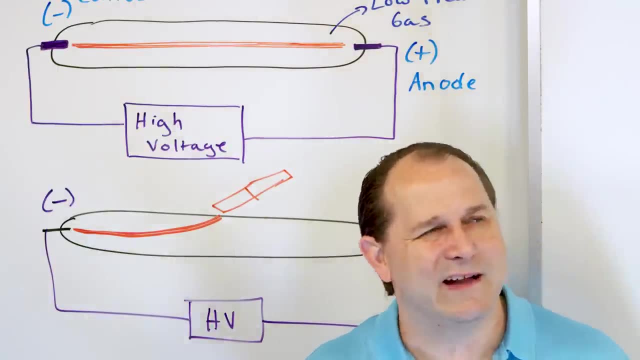 and so they were named the electron, and now we know that we call it a negative, a negative, one charge. it's a little bit arbitrary which particle is positive and which particle is negative, like why is the electron called negative? all we know is that protons are one charge and electrons are 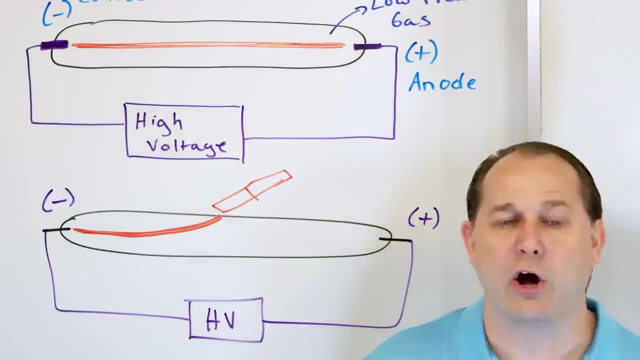 the opposite charge and we choose that the electron is what we call the negative species. all right now, the interesting thing about this is when you do the experiment over and over again and you put different materials in for the cathode, like maybe you put the cathode here made of carbon? 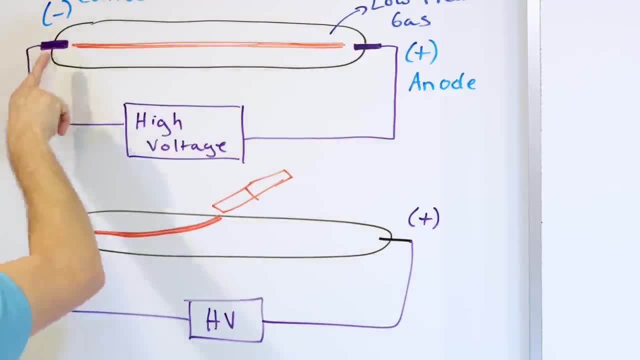 copper kind of sticking in here, and then you do it again with a gold cathode and you do it again with an alumina, you know whatever, whatever different kinds of conductive materials that are sticking into here. then it appears that the beam behaves the same way. the beam, the cathode. 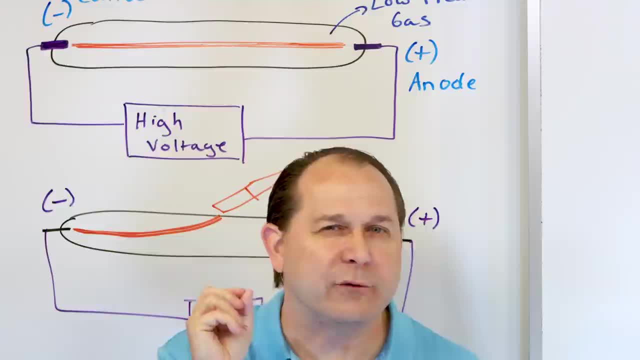 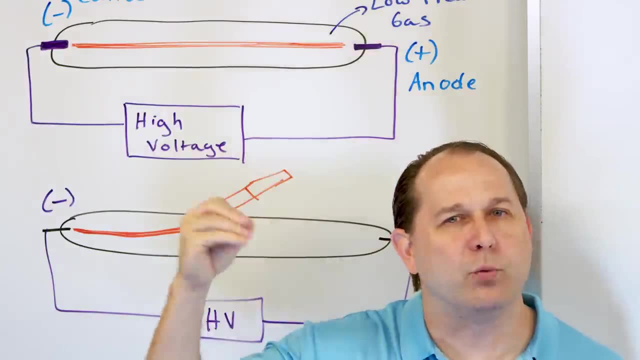 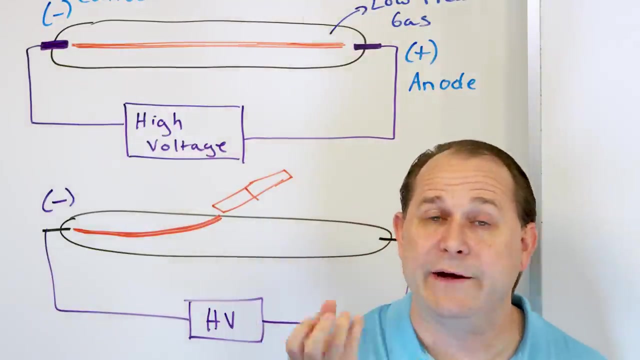 ray beam, which now we know is a beam of electrons, behaves the same way. that's a really big clue, because the beam appears to be exactly the same, no matter what different metal we put for the actual connection point on the circuit. then we assume that these tiny particles are emanating from the metal and they're always the same, no matter what. 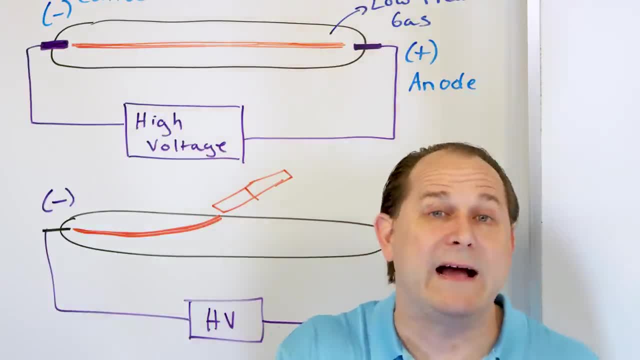 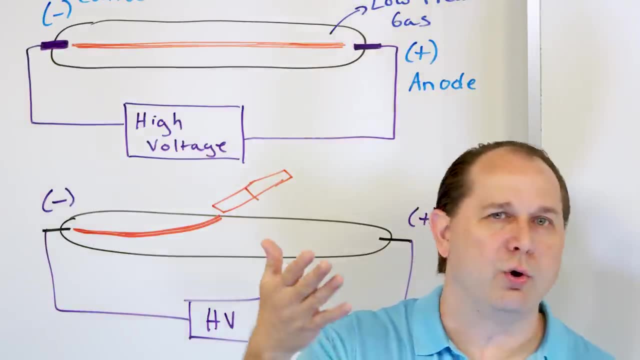 metal you put there, so maybe the metal is comprised in some way of these small particles which are then coming off, and that's exactly what's happening. so no matter if you put gold or silver or any other conductive material, the electrons that come off- we now know electrons. 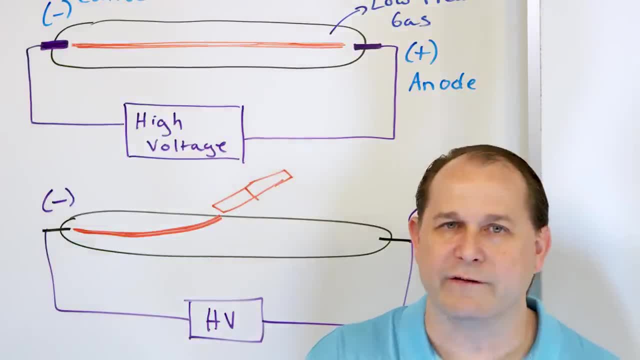 everything is comprised of electrons and we now know protons and neutrons as well. so it's no surprise to us, but back in the day it was very surprising that the beam would behave the same. so that was a big clue that whatever that that beam was, whatever those particles- 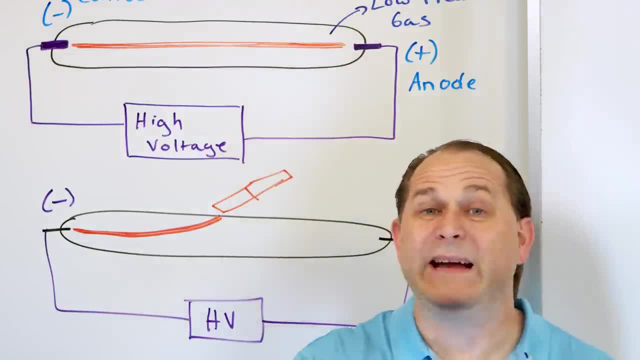 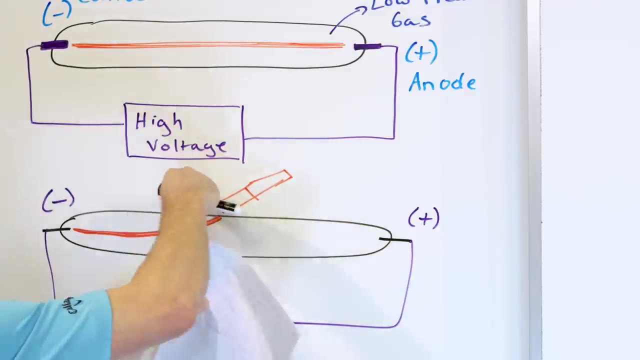 were those charged particles. they exist in many different metals, many different materials. okay, so then they said: well, wait a minute, maybe we can do some further experiments with this. we can generate this beam of cathode rays and um and we can influence them with magnets. and we can also put charge plates and influence them with charged plates. 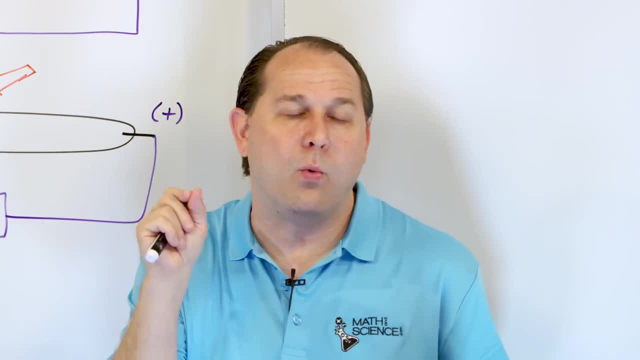 so let's do an experiment and try to learn more and more and more about what this beam of cathode rays there is around the region between a magnetic nucleus to a magnetic nucleus. so let's do an experiment and try to to learn more and more and more about what this beam of cathode rays really is. That was the goal. 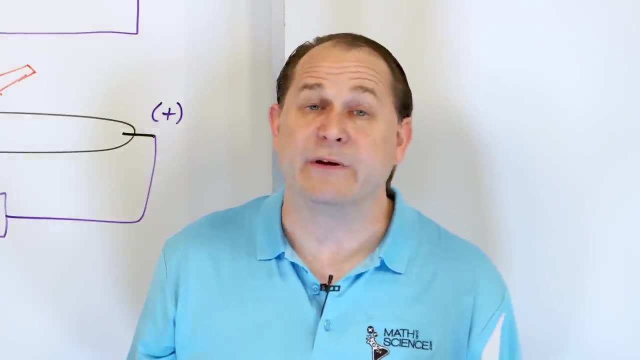 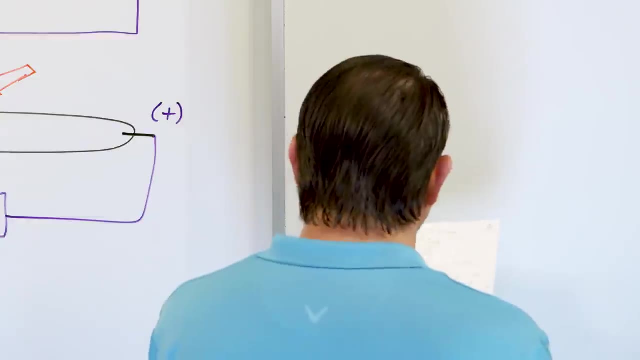 Let's see if you could figure out what these things are, because maybe it's a building block of the fundamental building blocks of matter, And of course we now know that is the case. So later on they built a similar version of this experiment. It's going to be difficult for me to. 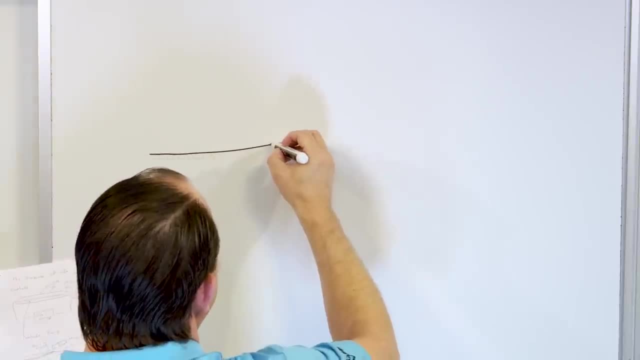 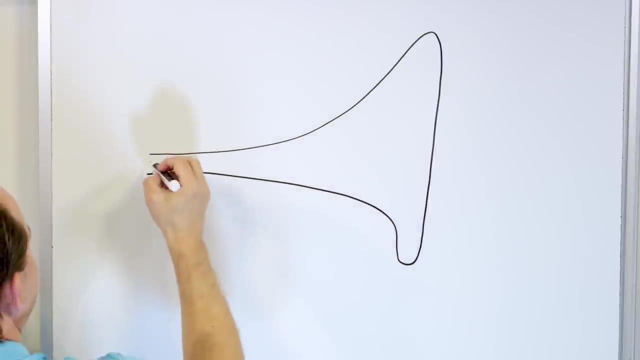 draw it because I'm not a good artist, but the basic idea is as follows: So they make another tube, but this one is shaped kind of like a horn or an ear, however you want to look at it, but it's a sealed tube, right, And this is a three-dimensional thing, So it looks kind of. 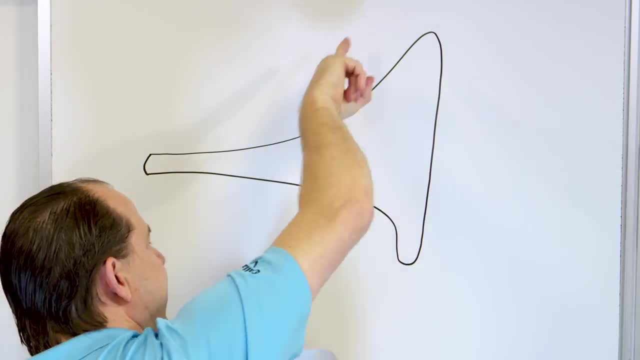 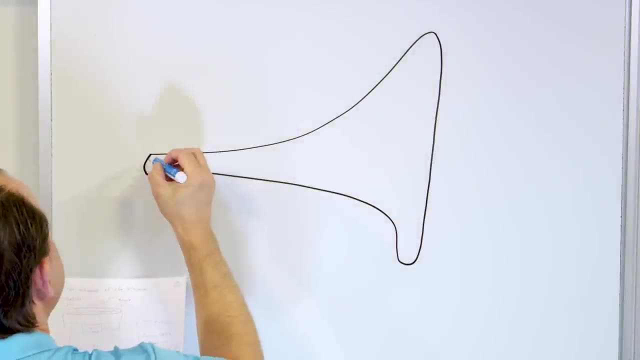 like a, you know, an outdoor light bulb or something like that. It's a circular thing at the end. then it goes to a small point like this, And what you do is over here. what you do is you inside of this thing. you put a connection point here to a cathode. I'll put a negative. 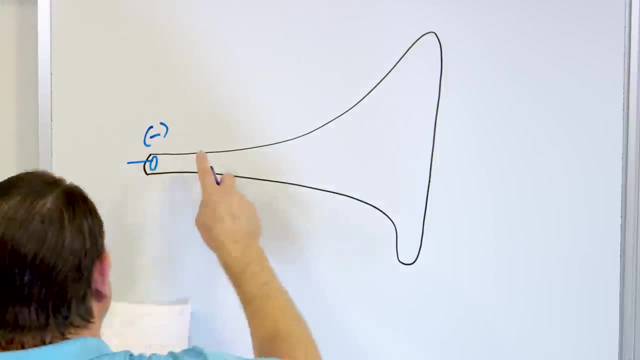 charge here, And then you put a negative charge here, And then you put a negative charge here, Object right there, And then down the way a little bit over here, you create an anode right here. But what you do is you put a hole in, you put a hole in the anode here. So what I'll call 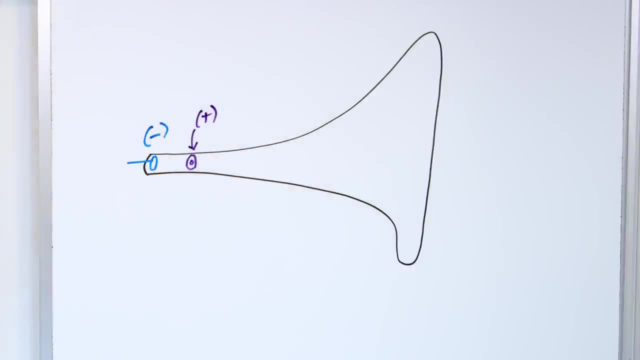 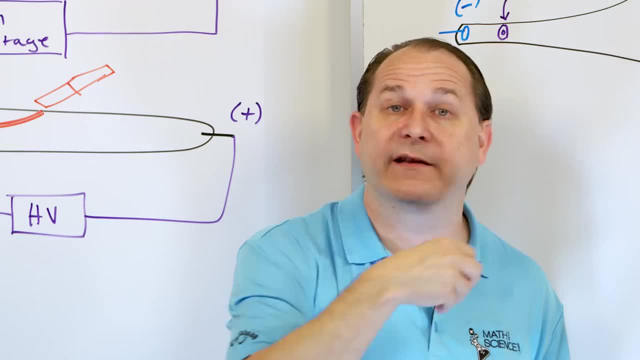 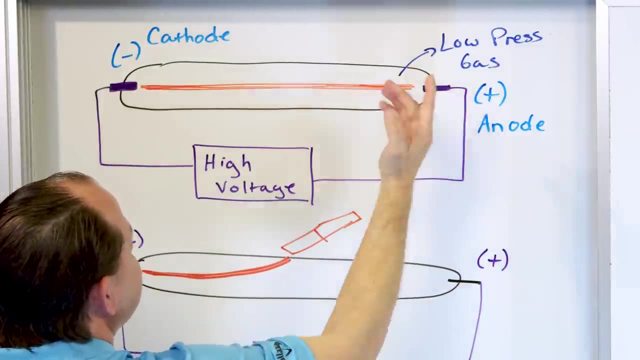 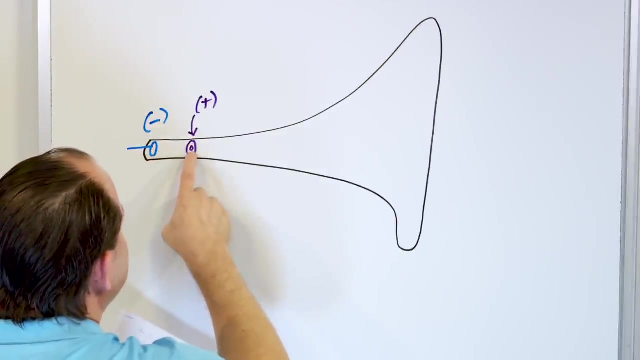 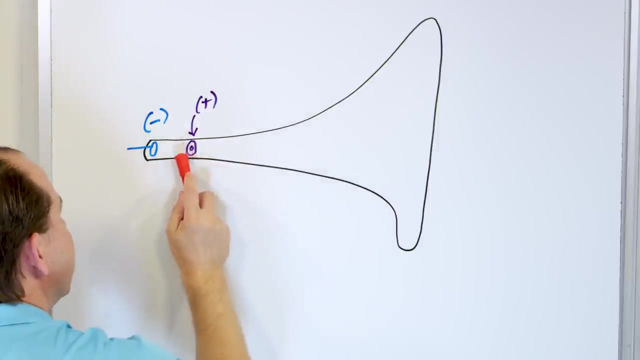 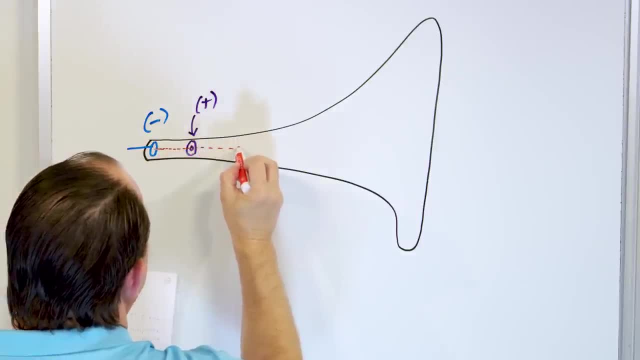 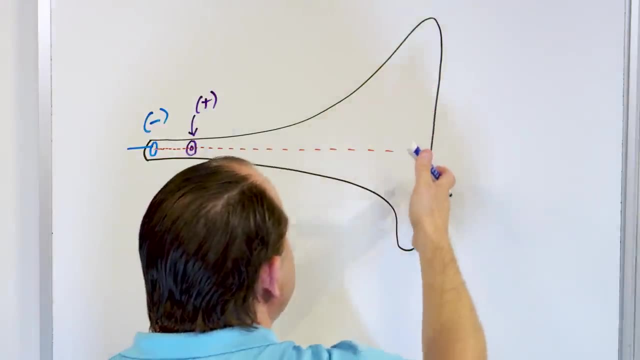 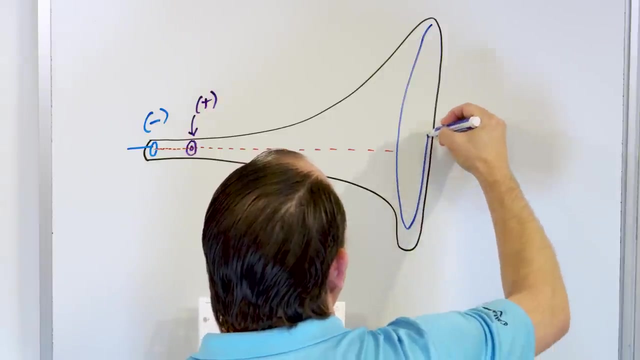 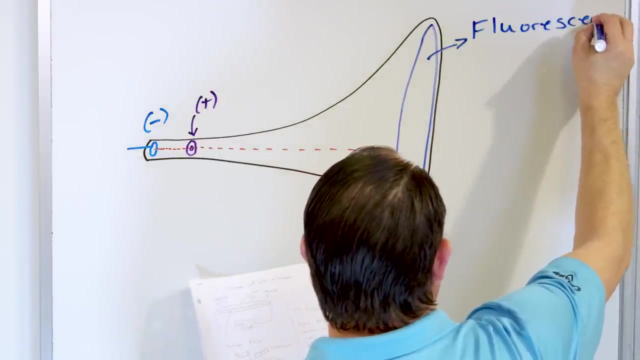 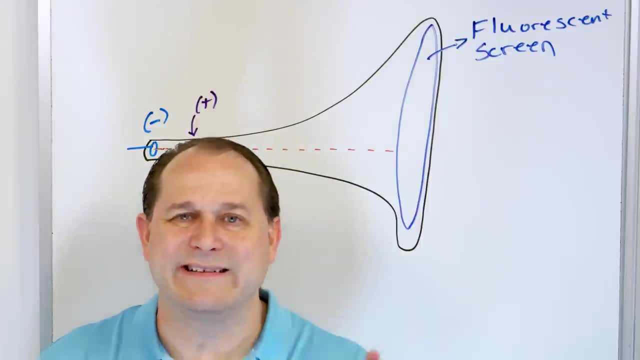 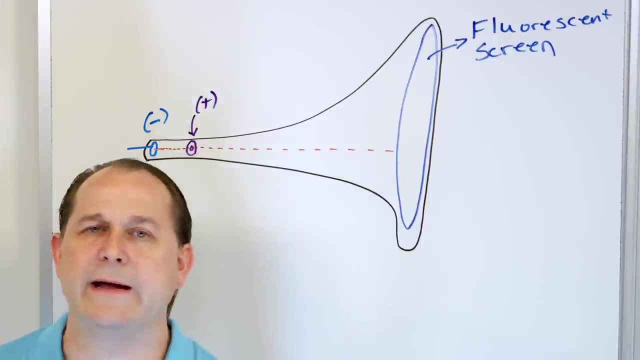 and painting the picture. So when you turn it off it glows for just a little bit there. Now, fluorescence is a whole other animal for a whole other lesson. But we were just talking a second ago that the red hot poker in the fire is glowing because the electrons are very excited from the 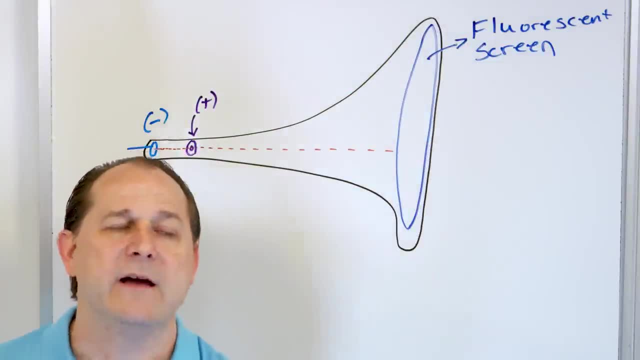 heat of the fire and they're going, bouncing up and down And when they decay they release photon And we see that as a red glowing poker. What's happening here is when the electron hits the fluorescent material, it kicks an electron up in the electron that exists in the in the fluorescent. 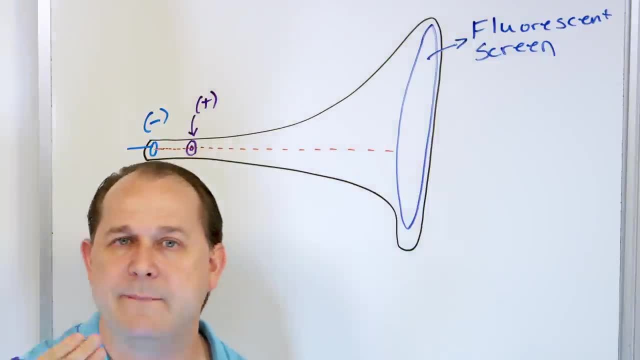 screen material And when that electron decays back down, it emits a visible light, because you can't see the electron beam. right, You don't see invisible beam of electrons, But what you do see is when the electron hits the screen it kicks an electron up which then decays back down and a 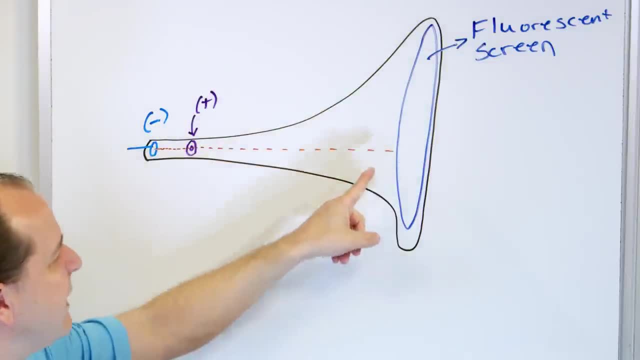 photon comes out And that's what you see. So this fluorescent screen allows you to actually visually see where the beam is impacted. The screen right And we can see that if you don't do anything else, this beam is going to go. 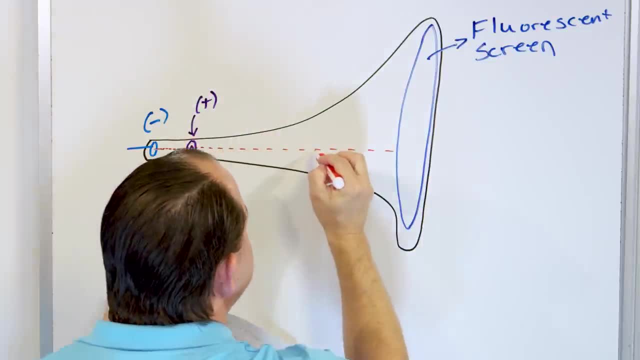 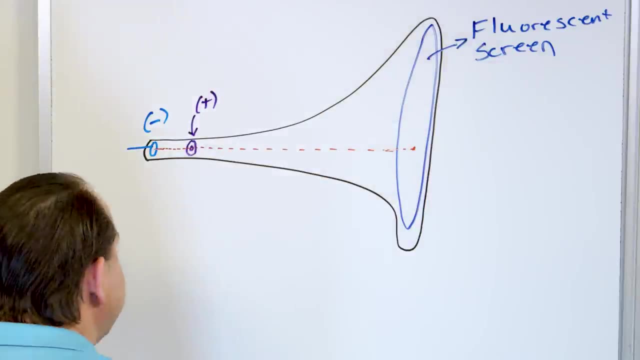 straight through the hole, accelerate it through the positive terminal and then it's just going to pick, it's going to go and impact And you're going to see a dot like right there on the screen. essentially, But if you want to learn what these, what these material, what these electrons are, 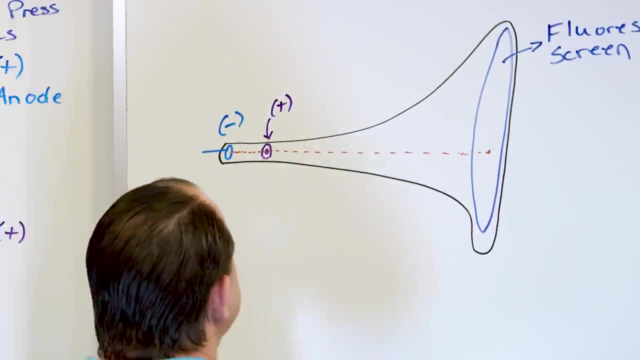 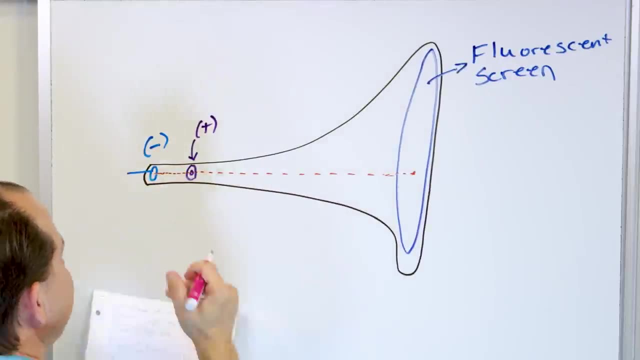 really made of. you want to play around with this beam and see if you can get it to deflect. We already said that we can get it to deflect with a magnet. So we and we also said verbally that we can get it to deflect with a charged plate. So what you do is 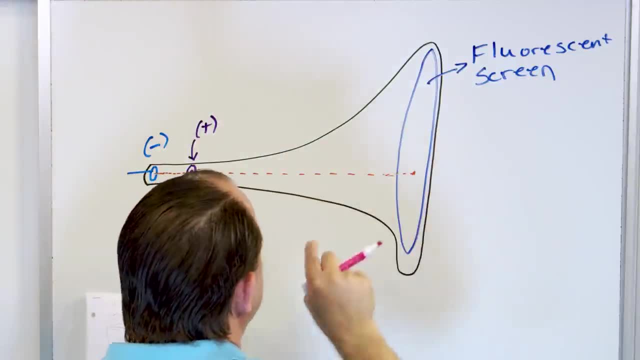 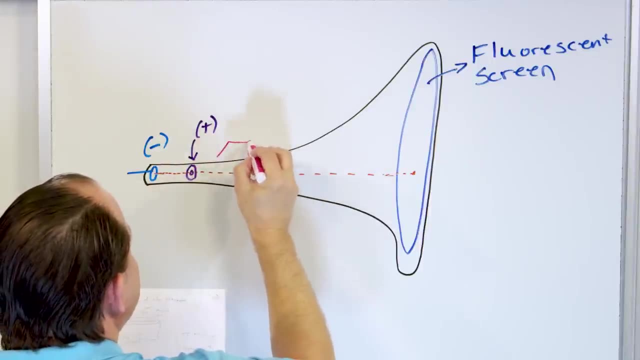 you have your electrons generated, they're accelerated through here, they hit the fluorescent screen and then just pass this positive terminal. What you do in the outside here is you put a positive plate or a or a charged plate on the top and a charged plate on the bottom. So this: 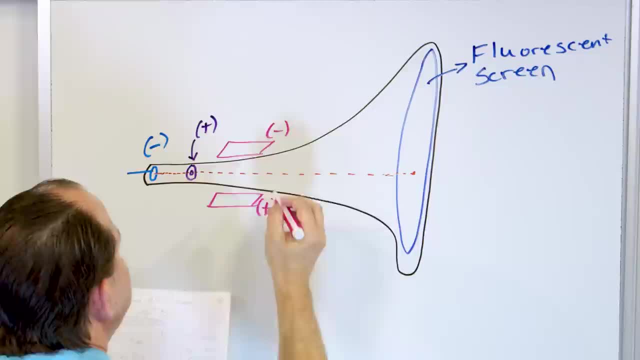 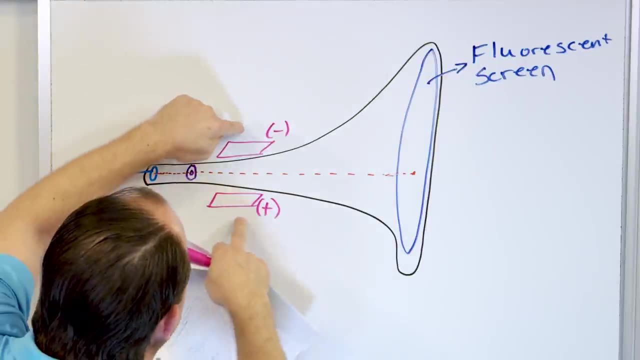 could be like the negative plate and this could be the positive plate And you have like a separate circuit that's going on outside here just to charge this plate up And you can. you can change the charges on here And when you do that, the beam is going to be bent up or down. 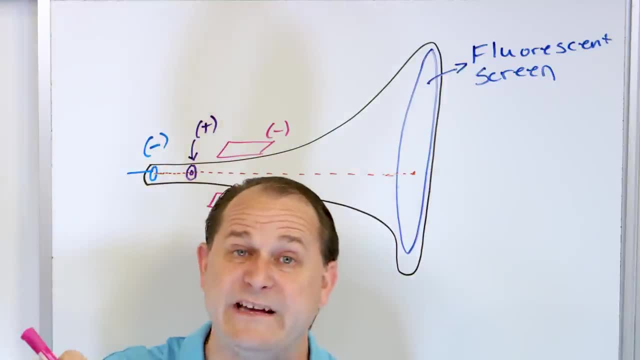 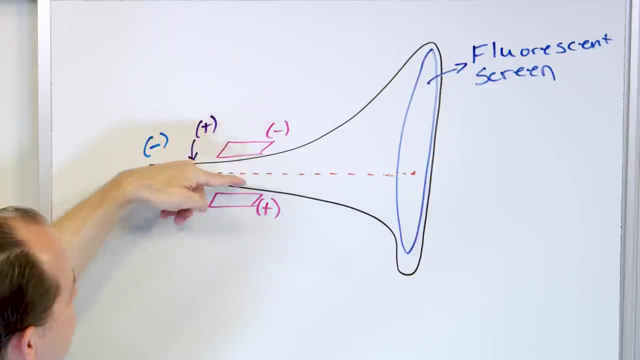 And, depending on how you orient the plates, you can get the beam to be steered, because the beam is, we now know, a beam of negative electrons, And so it's going to be repelled from this plate and it's going to be attracted to the positive plate And as you adjust the relative charges, 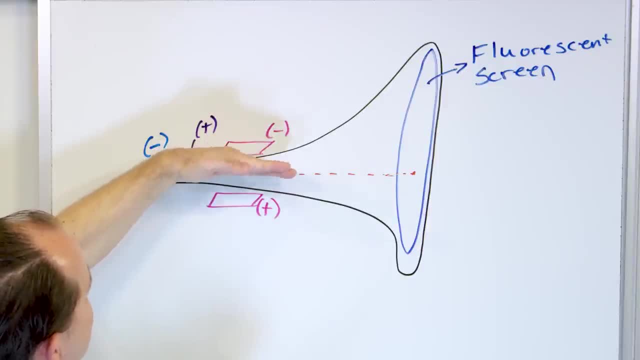 like, if you flip this one back positive, you can make the beam go up and so on, And so you can. that's how you can paint an electron beam on the inside of a TV, right? But then you go a step further and say, okay, I can bend the beam like this. Now, here's the thing. 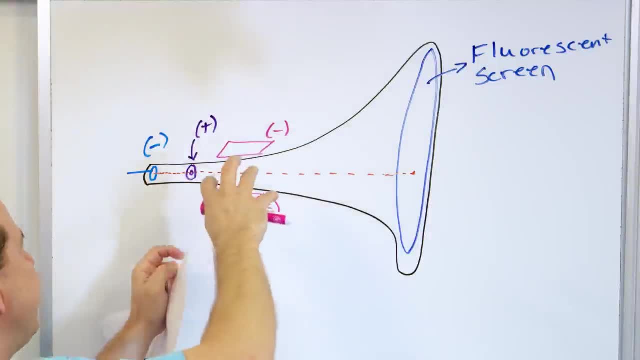 I cannot draw this without totally messing up my drawing, But if I, if you can visualize a plate on the top and a plate on the bottom, that is an electric field that's moving the beam around. If you can visualize another electromagnet which is here and then it wraps around to the other. 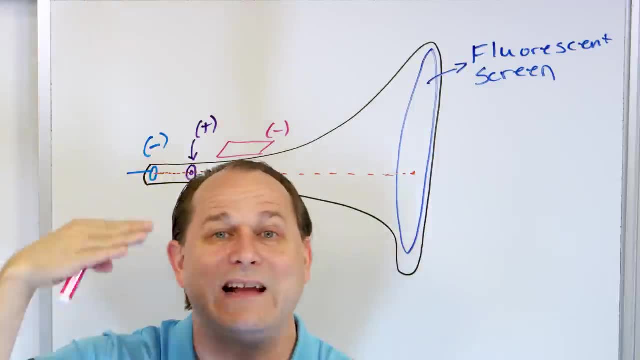 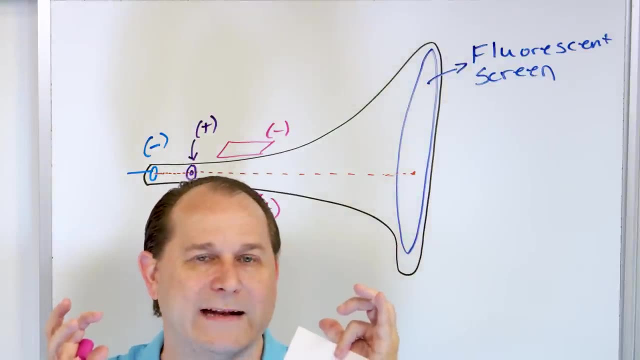 side. So there's electrical plates which are using the electric field to steer the beam And then, perpendicular to that, you can see that the electric field is moving the beam around. You have kind of a bar magnet going all the way around, but it's an electromagnet. 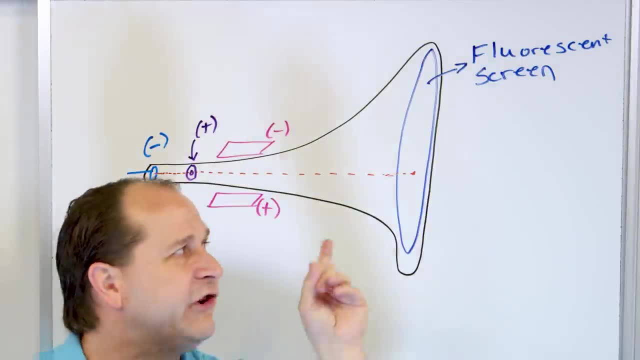 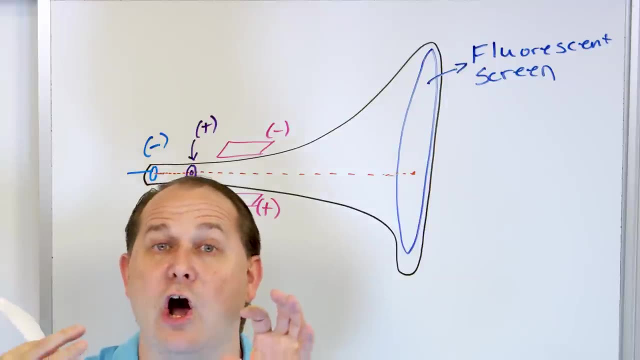 that you can also change the intensity of. So you can change the intensity of the charge plates to steer the beam And you've you can construct this magnetic field also to steer the beam And you can get those two to exactly cancel each other. So what you can do is you can say: 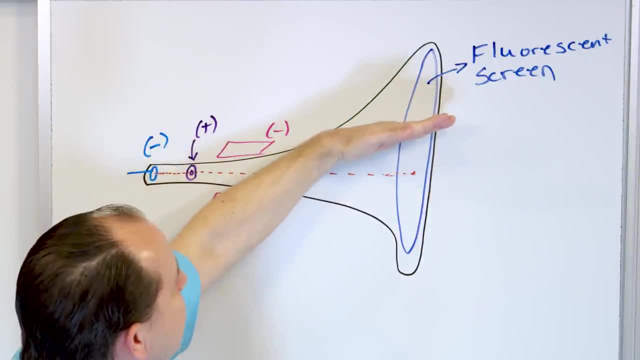 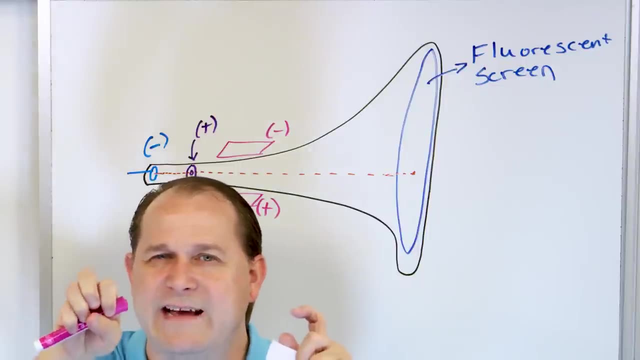 all right, I'm going to turn these plates on and get the beam to slant up and hit the hit the screen right here. And then I have these magnets which I can also adjust, And I'm going to turn. I'm going to turn the magnetic field exactly to bring the beam back down and make it go straight. 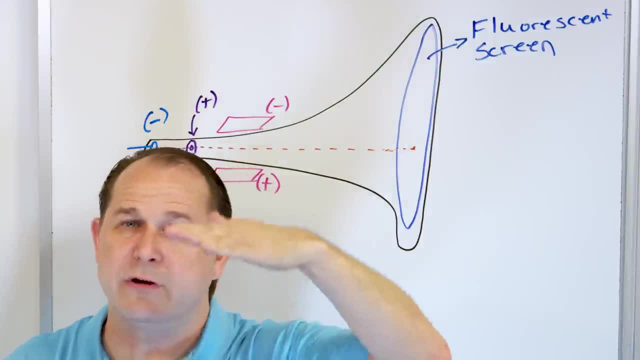 again. So because you know how much you've deflected it and you can measure that and then you can adjust the magnetic field to exactly counteract that and make it go straight again, Then you have all the information when you do a bunch of runs of this experiment to figure out. 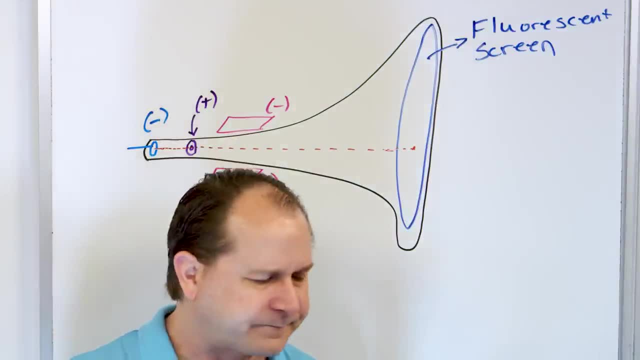 how much charge must exist on this electron right? Because that's what you're trying to do. They didn't really know what the charge actually was on the electron, And so they wanted to do these experiments. Now it turns out that you can't. you don't have enough. 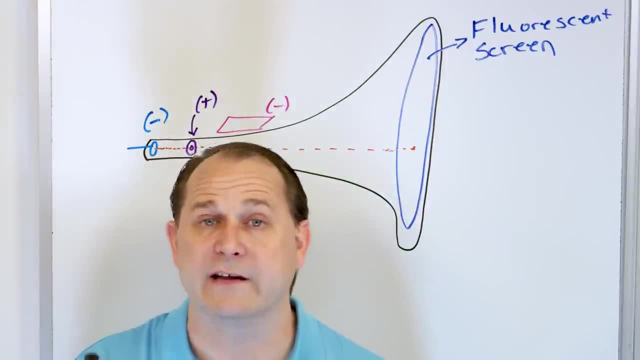 information to figure out exactly the absolute charge on the electron. but what you can calculate is the charge on the electron divided by its mass, the charge to mass ratio. So when you do these experiments, adjusting different electric fields and canceling them by the magnetic field, and you 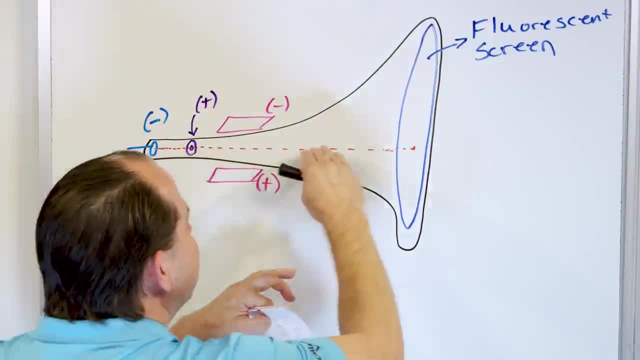 know how, the strengths of all these things that you need to to set up to get the beam to go straight. What you figure out is that for an electron, you have 1.7,, you have 1.7,, you have 1.7,. 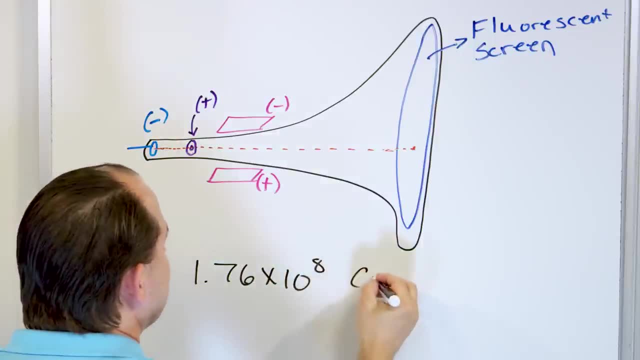 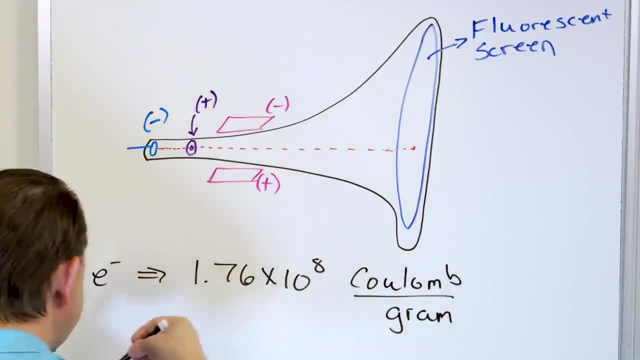 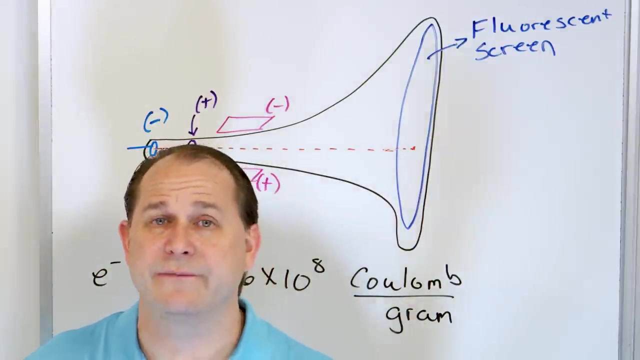 6 times 10 to the positive eight coulombs. I'll talk about this in a second per gram. Now, the coulomb is something we haven't talked about. That's a unit in physics and also in chemistry. It's the unit, the SI unit of of charge, of any kind of charge. All right, It's a. 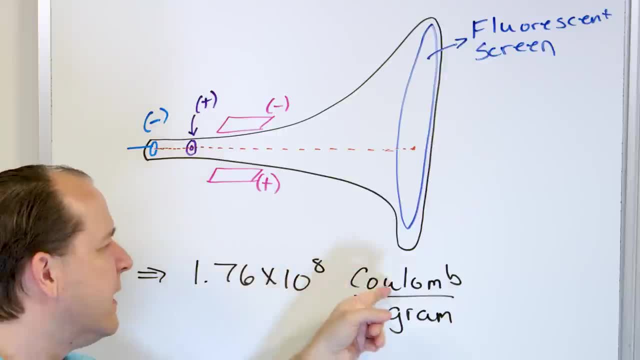 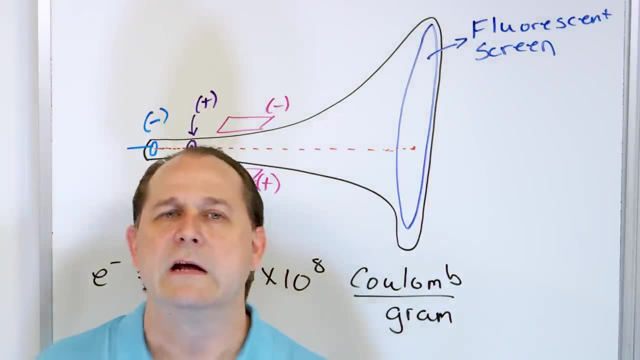 it's a very, very, very. you know, this is a very, very small- or I shouldn't say small, It's a, it's a unit that we use to talk about the charge of the electron, the charge of the proton, the charge of ions. It's, it's something that you're going. 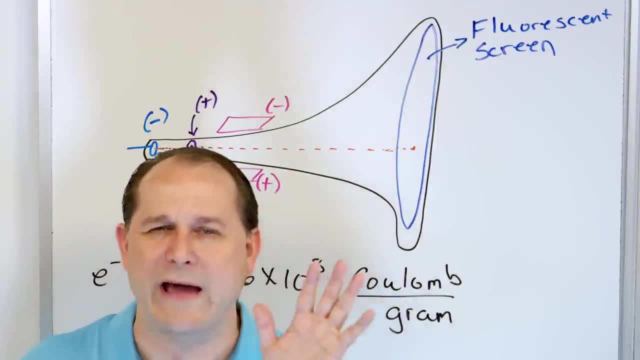 to get used to using as we go on. For now I don't. I know we haven't done any calculations with coulombs yet, but for now just know that when you do this experiment you can calculate 1.76 times 10 to the eight coulombs per gram of the electron. So you don't know the charge in the. 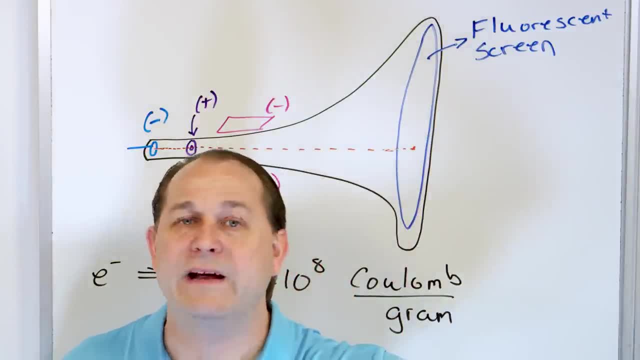 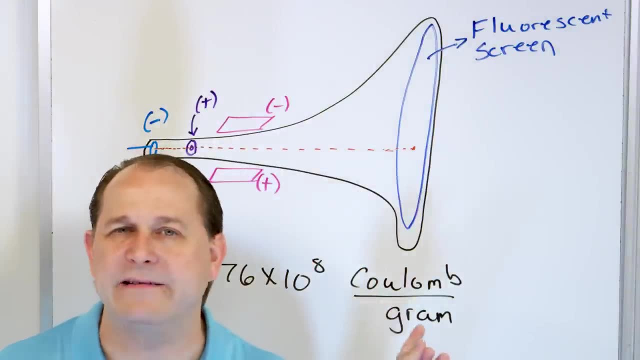 electron. What you know is the charge on the electron divided by whatever its mass must be. So ideally you want to know what is the charge of the electron and what is the mass of an electron. This kind of bakes all into one unit. It's that many coulombs of charge per gram of the electron. but we don't. 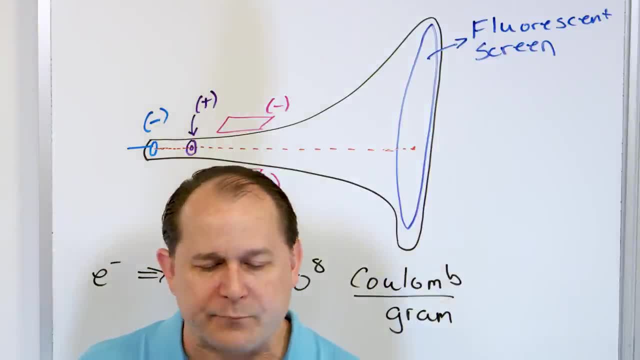 know exactly how many grams an electron is. So it sat like that for a while And then, several years later- because this is right at the turn of the century, the turn of the 1900s, right. So we started to understand how much charge per unit mass an electron, a single electron, would. 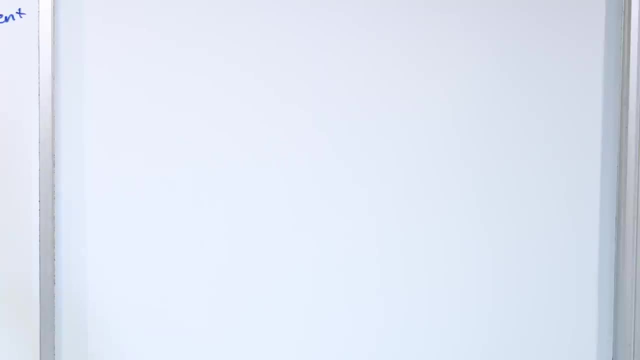 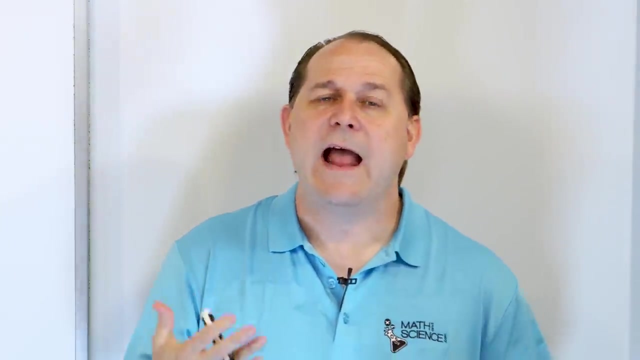 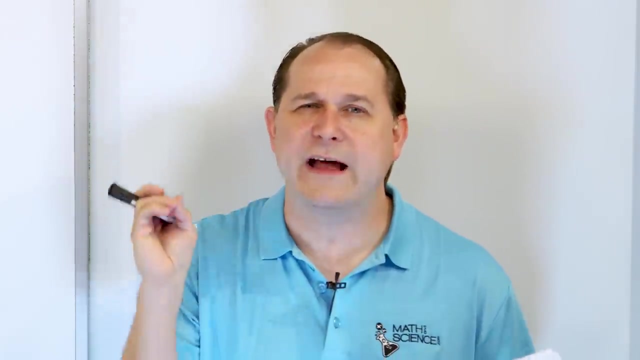 have. Then, in 1909, a famous experiment called the Millikan drop experiment was conducted, And that purpose of that experiment was to determine the exact charge on the electron, right To see if you could figure out what is that charge on the electron. 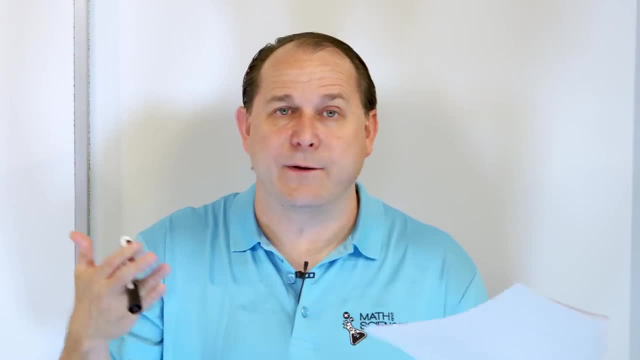 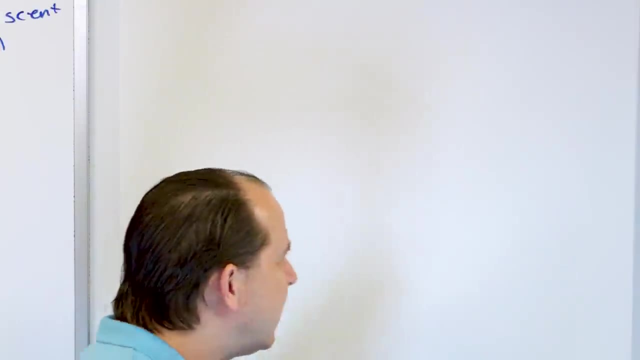 because everybody knew. now that you know this, cathode rays were electrons, We want to learn as much as we can about them. Probably the most important thing we can understand is: what is the charge? So a clever experiment using drops of oil was constructed, So I'll try to do my best. 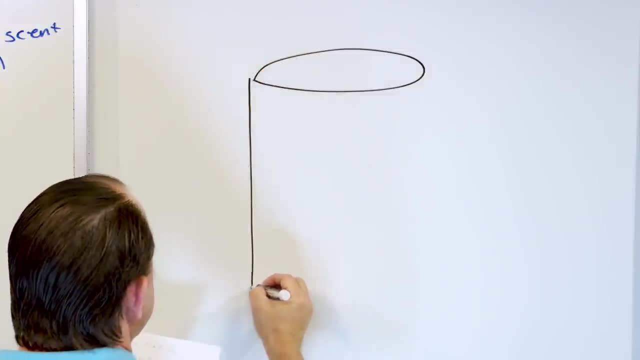 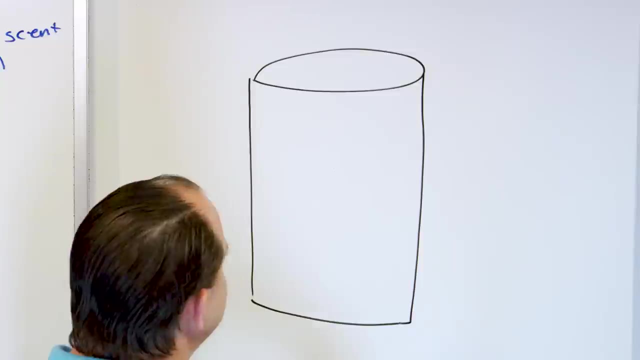 It's not going to be perfect, but basically here is like a drum and I'll kind of come down here and draw it like this. And honestly, when I look at this, when I look at how he set this experiment up, I'm kind of in awe that somebody would even conceive of this And then to be able 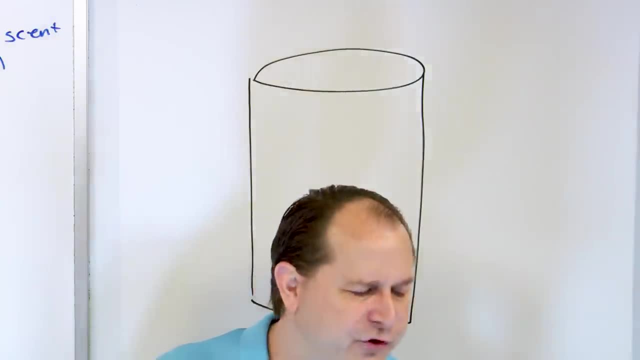 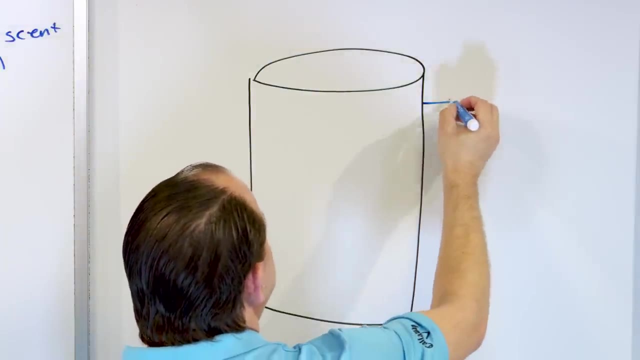 to have the precision necessary to do anything meaningful with it and to do it in 1909, that's crazy to me, but this was done right. People are people are ingenious, right. So what you do at the top here is you inject into the top of this vessel oil. I'm not exactly sure what type of oil he used. 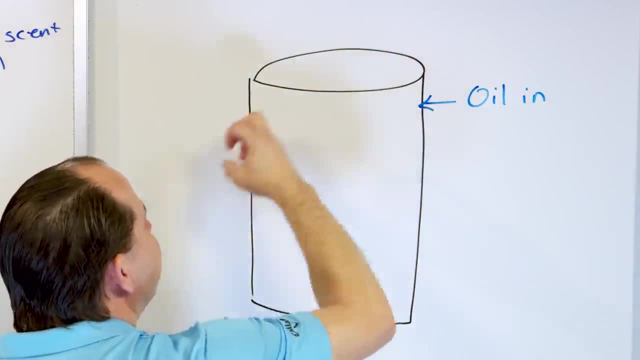 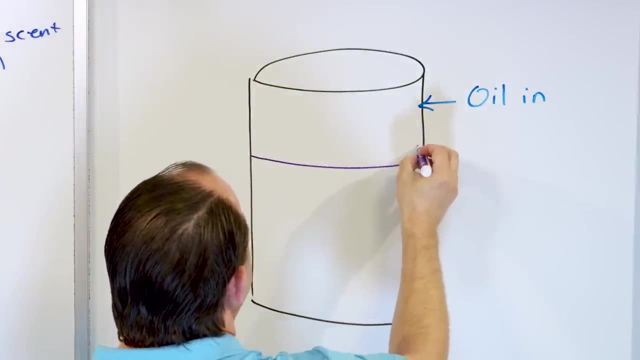 but you can inject oil into the very top. You can spray it into very small droplets. So then, the way this thing was constructed is there was a plate right here at the top, like this, with a hole in it right here, And so you inject this. 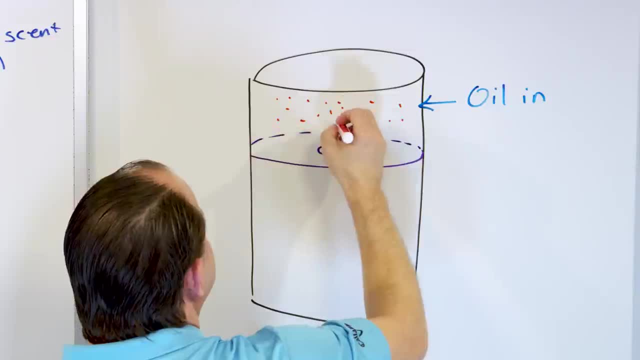 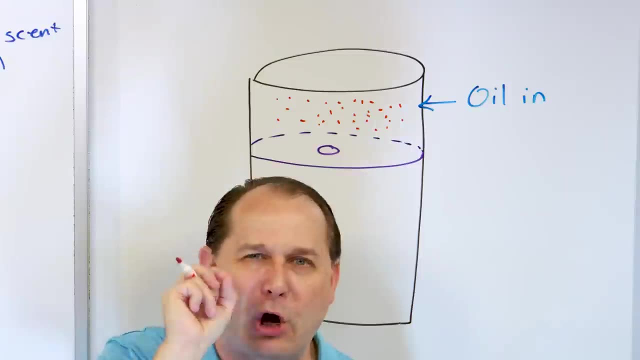 oil in the top and you and you inject it in a very fine mist like very small micros. I'm not talking about giant droplets or gobbles of oil, I'm talking about microscopic particles of oil- Uh, so small that you can't almost even see them. And what they do is they go And, of course, 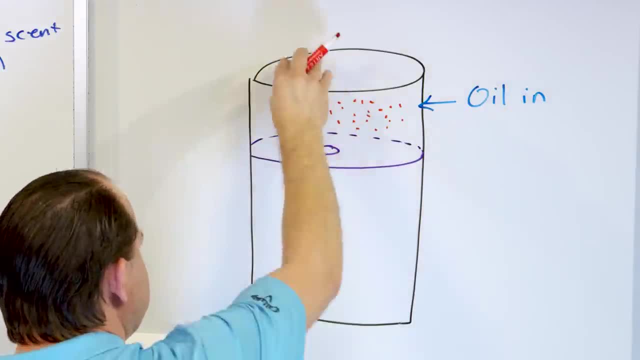 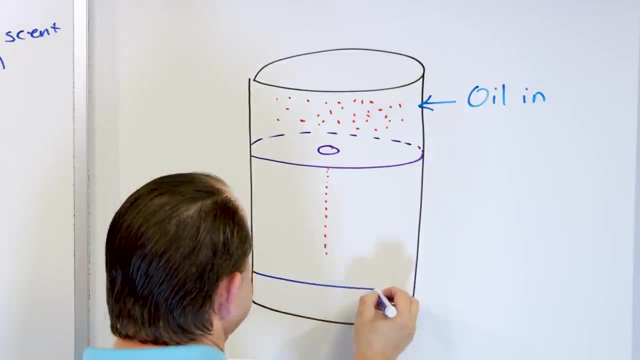 there's this hole there, So they begin to kind of like go down, kind of in a straight line through this hole down towards a another plate which is located here at the bottom. I can do this, something like this: All right, Now these plates are charged, because we know electrons are charged. 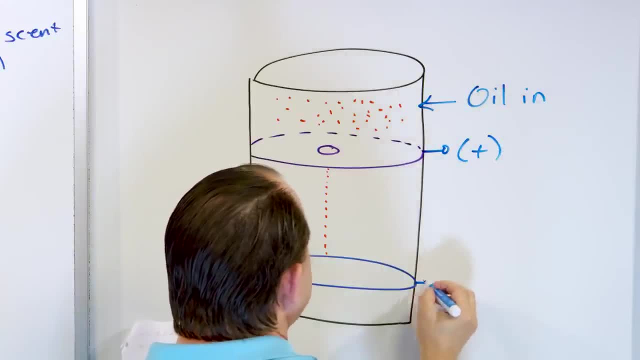 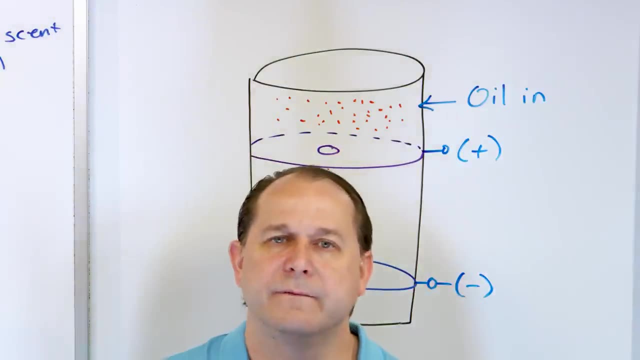 And so we charge this plate up with a positive charge and we charge this plate up with a negative charge. All right now. oil by itself? Uh yeah, everything has electrons inside of it, but because there's protons in the center of the nucleus and electrons on the outside, equal and 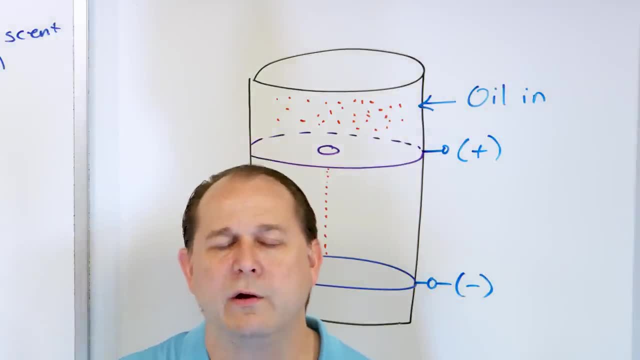 opposite charges. most matter around you, including oil, doesn't have any observable charge from the outside world. It's kind of crazy that everything is consisting of these charged things, but we don't notice it because there's always equal and opposite amounts of protons and electrons, right? 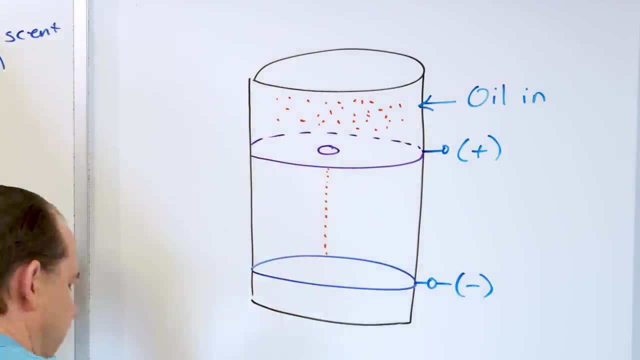 Same thing with the oil. So the oil is just. this thing is coming down like this. but what, uh? what they did is they then connected an x-ray machine and put x-rays into this, uh, into this vessel. the x-rays impact the oil. 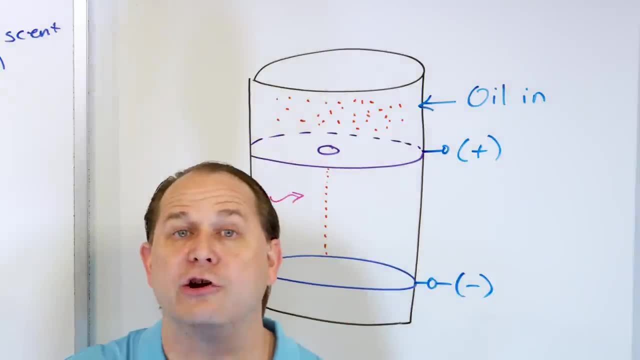 And when the x-rays hit the oil, they basically put a charge uh on on the oil, or they they make, they force a net charge to happen on the oil droplets. The details of how that happened aren't that important, but basically what you can do is you can make the oil charge. So it's. 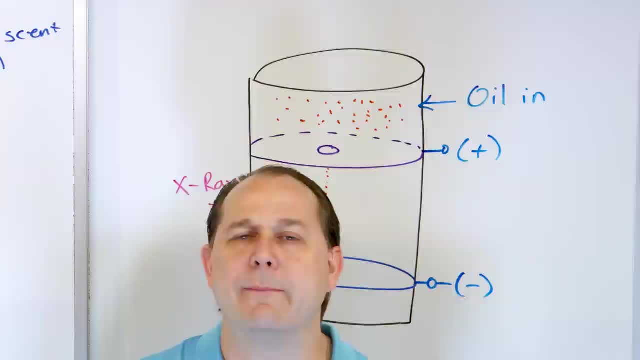 no longer a neutral atom atoms uh that are in there in the oil droplets. it's charged uh uh you, because it has a net uh, net uh uh. charge on the oil droplets Now, since the oil is. 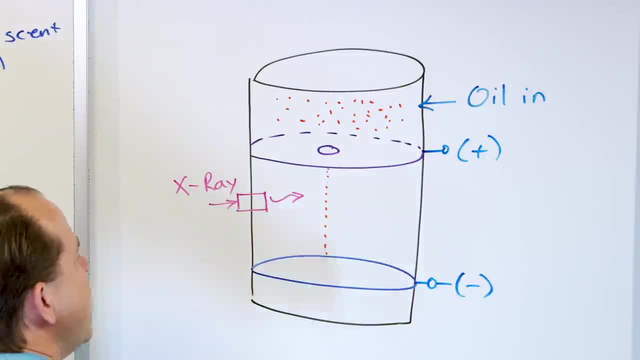 microscopic and they now consist of having a charge on them. you can adjust the positive and negative terminal here to exactly cause the oil wants to fall down due to gravity, right, And you can then adjust the charge on the plates to exactly counteract the force of gravity. So 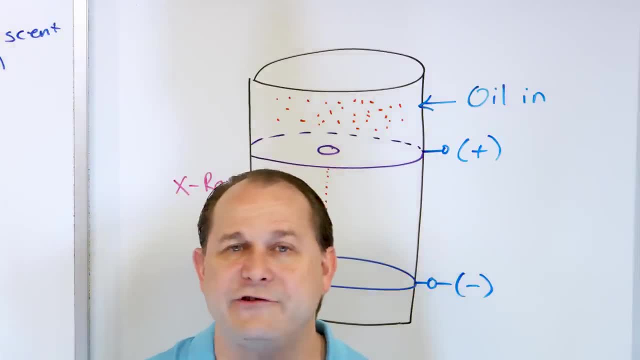 everything wants to fall down. We know how things like to fall- acceleration of gravity in Earth's gravity as a constant thing- So we know that the oil should take a certain amount of time the tiny little drops to reach the bottom. Now that they're charged we can adjust. 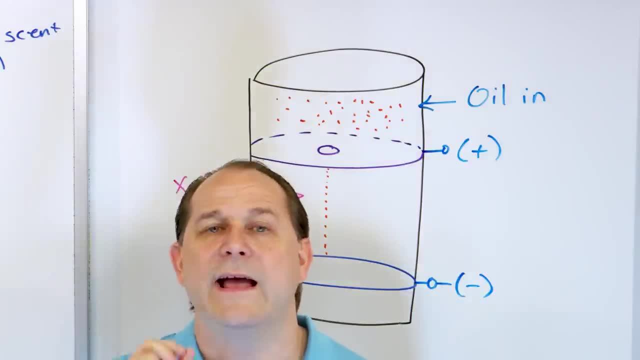 the plates to exactly cause them to no longer fall anymore, And then we can know how or what the charge on the oil is. And from all this, uh, I'm very much simplifying it. I mean, this is, this is a crazy clever experiment to actually figure this out. Then it was figured out that 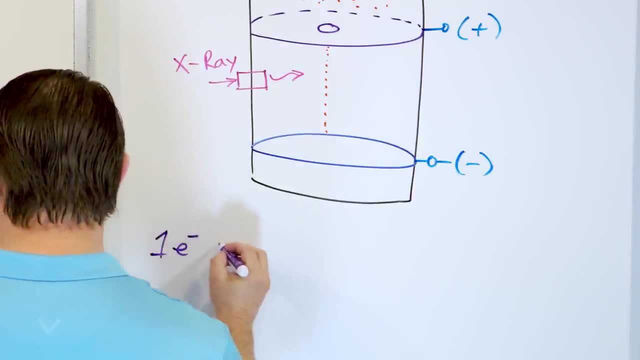 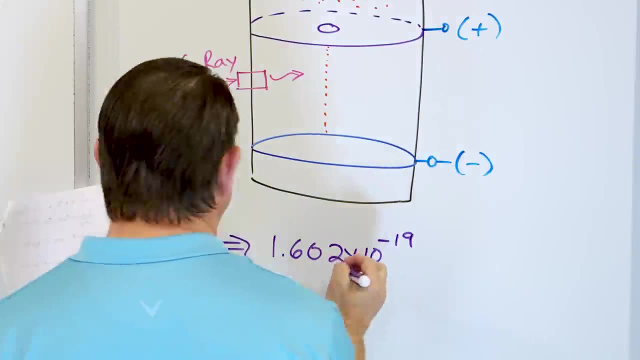 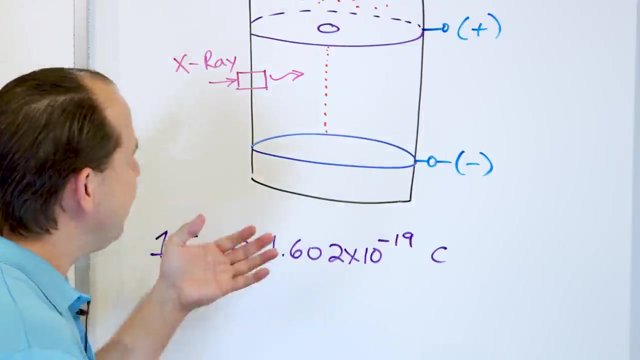 the charge of a single electron must be equal to 1.6,. Oh, two times 10.. To the negative: 19 again in the unit- uh, this is six zero two, Sorry about that- Uh, the unit of Coulombs, which is the unit of electric charge. Now I am. I'm skipping over a lot of stuff, because 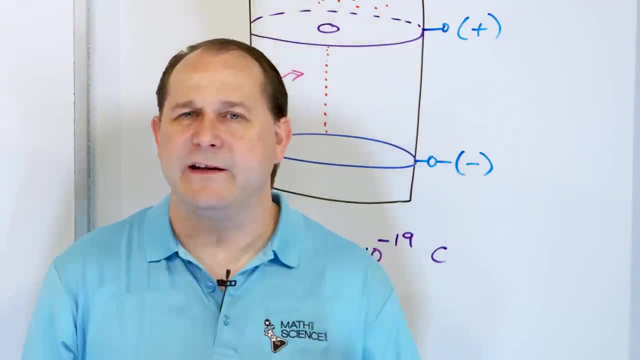 I mean, um, there's just a lot of details in an experiment like this, And of course he did back in the day. Uh, it's not so simple, Like there's a digital readout and it says: here's the charge. 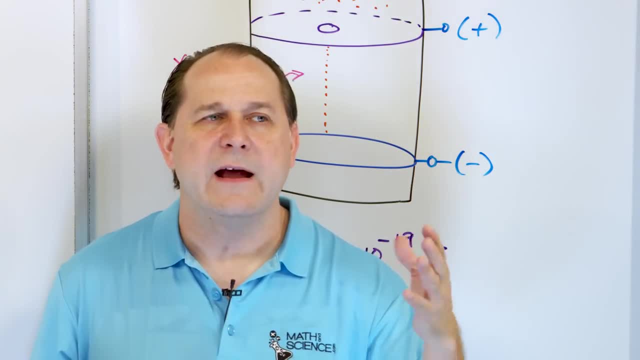 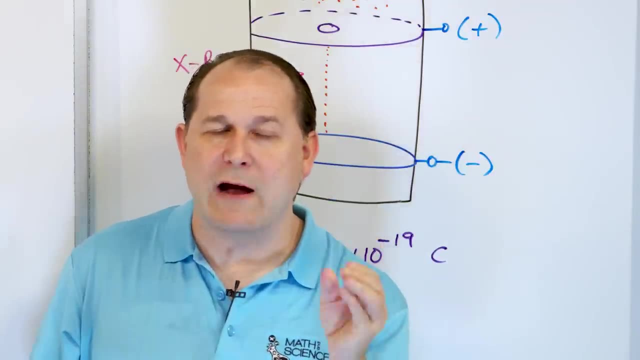 It doesn't work like that. What you do is many, many, many runs And you figure out that the, the charge on the drops, is always a multiple. The, the charge on these large drops, which are much larger than an Adam, is always a multiple of this number. So because 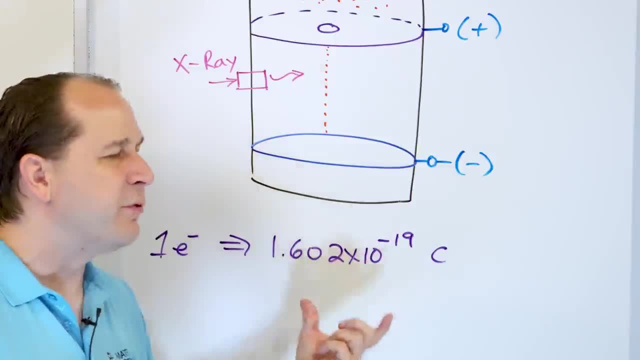 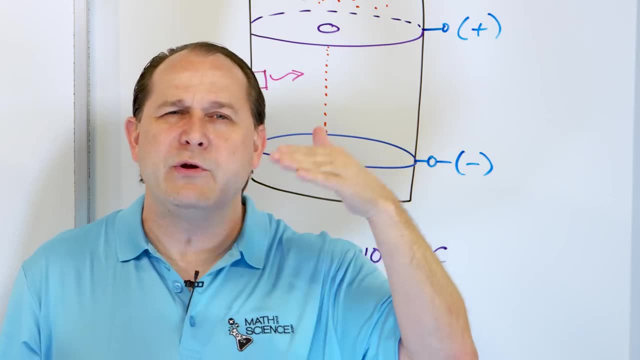 the charge is never smaller than this and it's always a multiple of this number, then we deduce that one of these little electrons must have this as a unit of charge, because this is the common multiple. I mean, when you, when you excited oil, uh drop it like that with an x-ray, it's not. 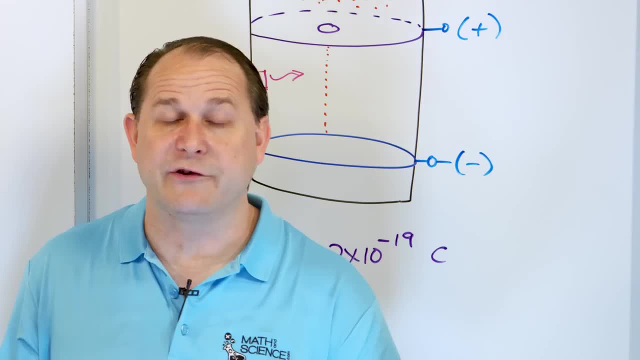 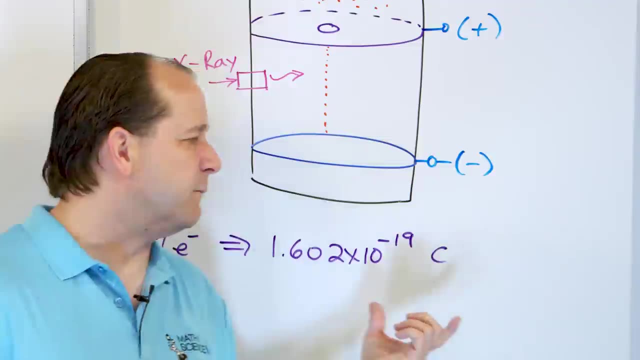 going to pick up like one electron. It's going to have some multiple electron, uh electrons that are either knocked away from it or added to it, Right, And it turns out that the multiple is a multiple of this number. So they deduce this must be the charge on a single electron. Now, 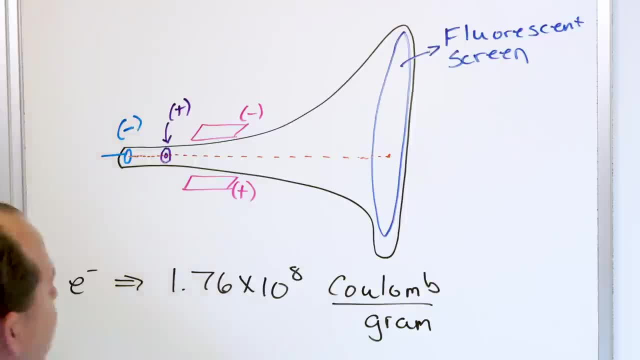 here is where it gets. in my opinion, really awesome, because before from a totally different experiment. when we accelerate a beam of electrons and we can deflect them with a charged plate and then we can use magnets- which I didn't draw- to counteract that, Then we can deduce that the 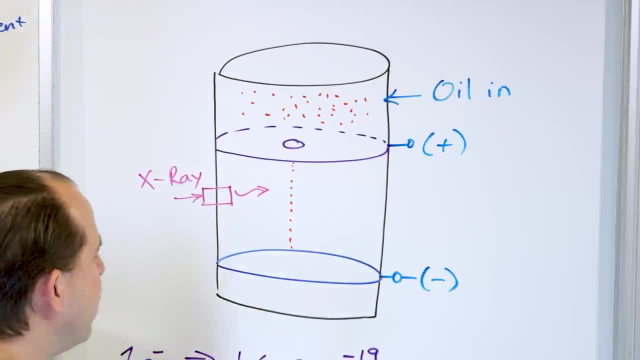 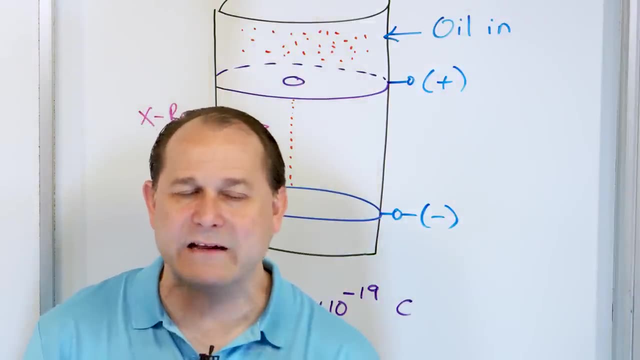 charge per gram must be this, And then, from this experiment, we now know what the charge of an electron is, And so by putting those two pieces of information together and the power of dimensional analysis, which I've been telling you is, like, so important, you can calculate actually. 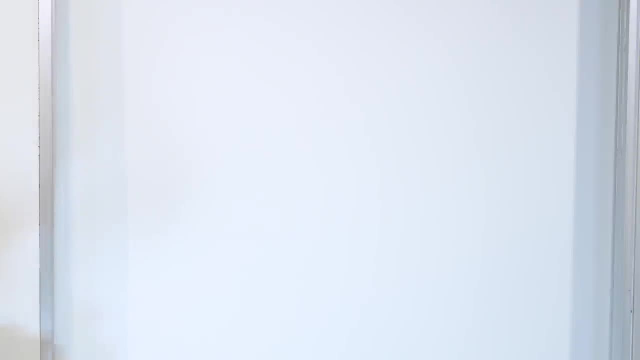 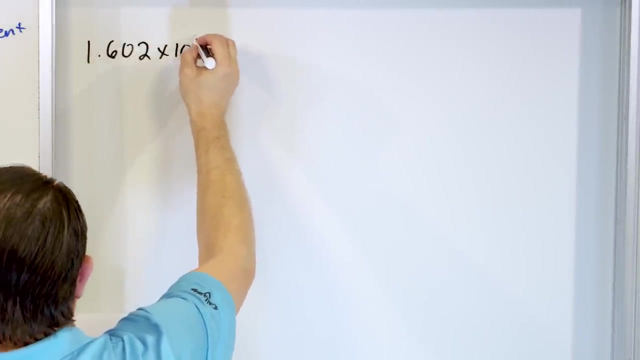 what the mass of an electron is, And we're going to do it right over here. If you start off by knowing the number I just wrote down: 1.602 times 10 to the negative 19 coulombs. This is just. 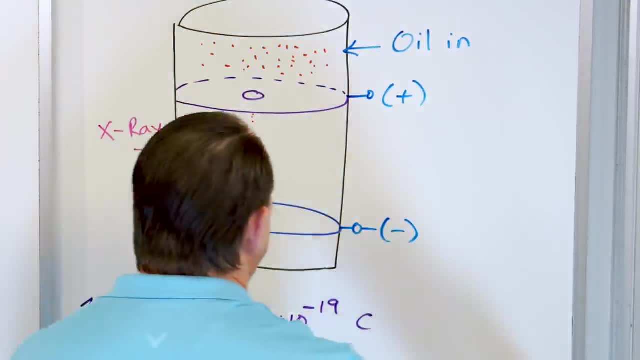 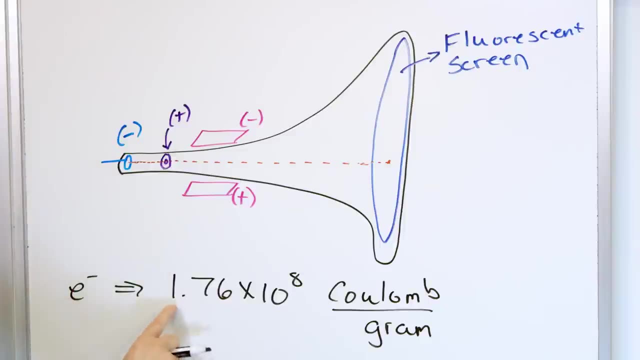 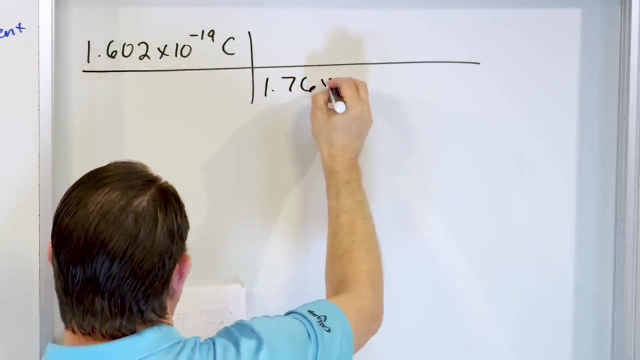 this is the charge. I exactly wrote it down from the Millikan oil experiment, right? And then we go over here and say, all right, what else do we have here? We know that it that the electron is 10 to the negative 18 coulombs per gram. We want to write it like this: 1.76 times 10 to the eight. 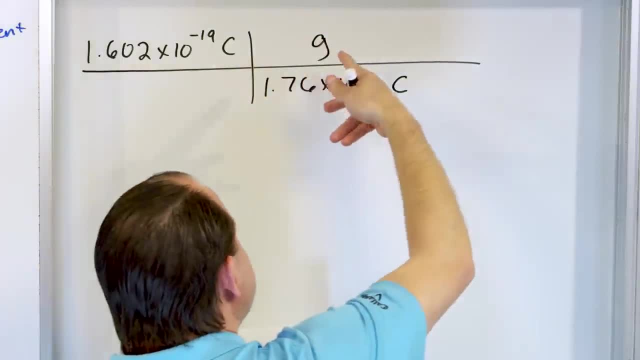 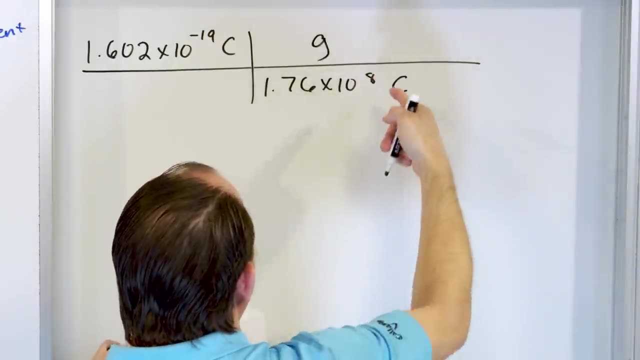 coulombs per gram. Remember anything in an in a unit conversion. you can flip it over either way. It's coulombs per gram. You can write it coulombs on the top and grams on the bottom, or coulombs on. 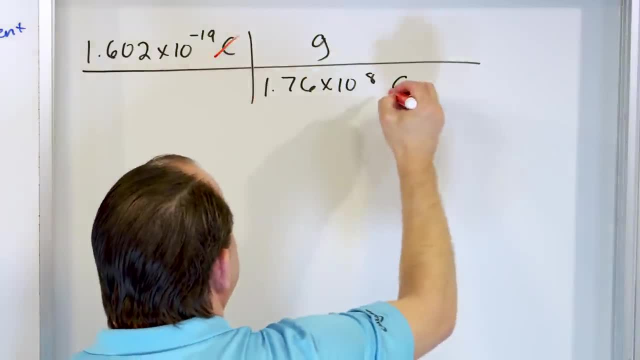 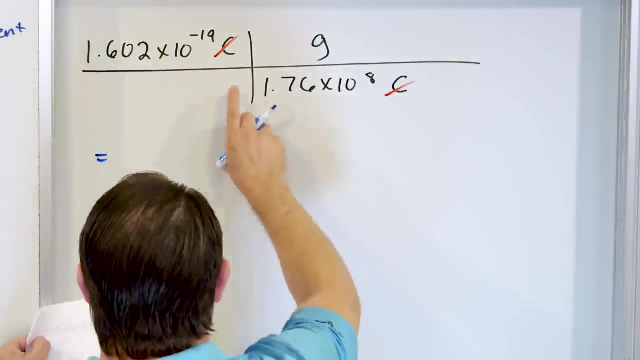 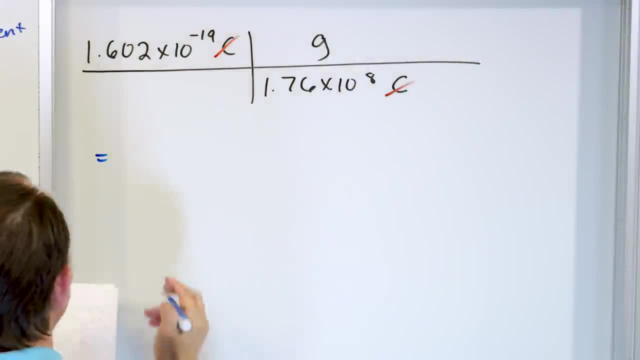 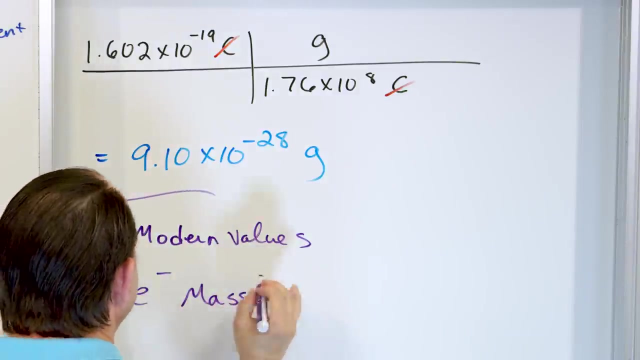 tiny number, don't forget, and divide it by a really, really big number. What do you actually get? 9.10 times 10 to the negative 28.. And this is grams. Now, this was a value calculated in the early 1900s. right Now, what about modern values? Right, The electron mass, the modern accepted? 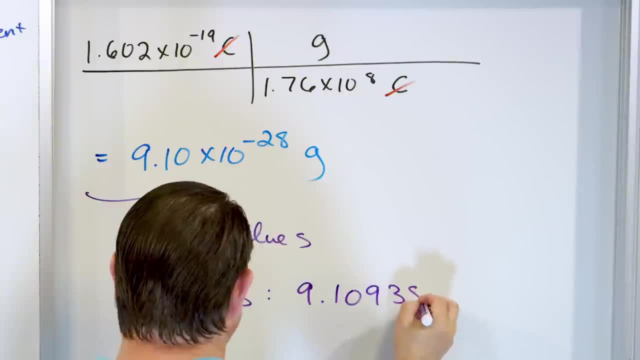 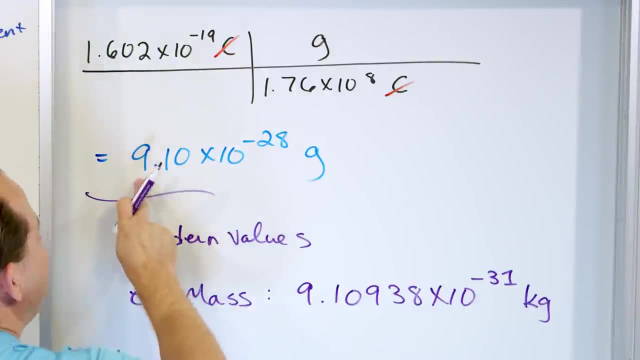 value for it is 9.10938 times 10.. So the negative 31,. but the unit we use typically in calculations is kilograms. Notice what he calculated was 9.1 times 10 to the minus 28 grams. But if you want to take grams to kilograms, 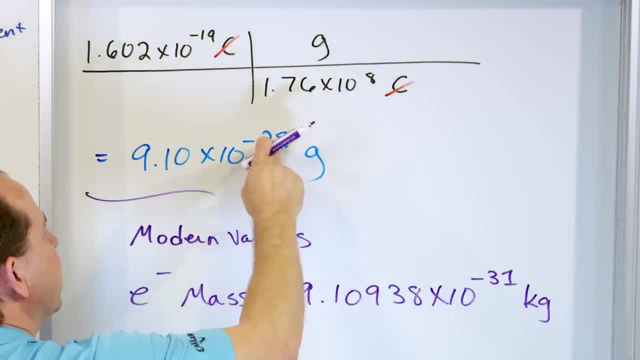 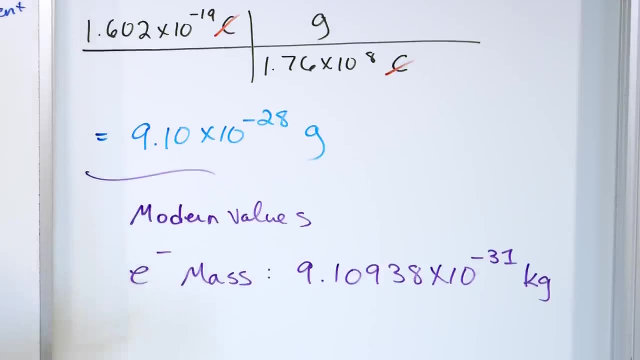 you need to divide by a thousand, So that's going to make this three. It's going to be subtracting three from the exponent because you're going to move the decimal three spots to the left. That's why it's a negative 31 kilograms. And then the electron charge. 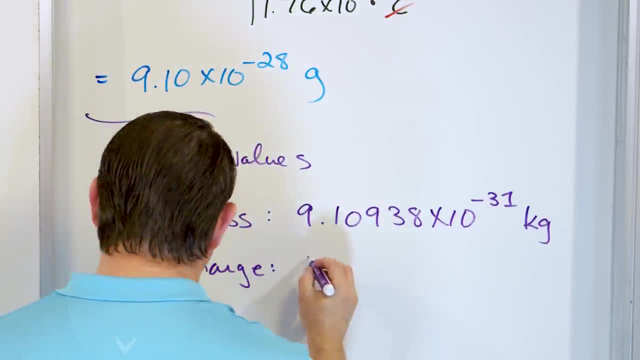 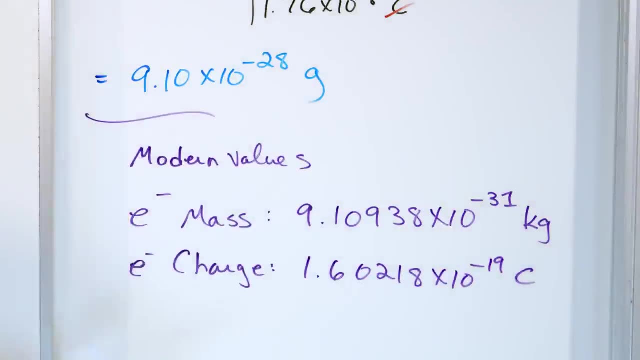 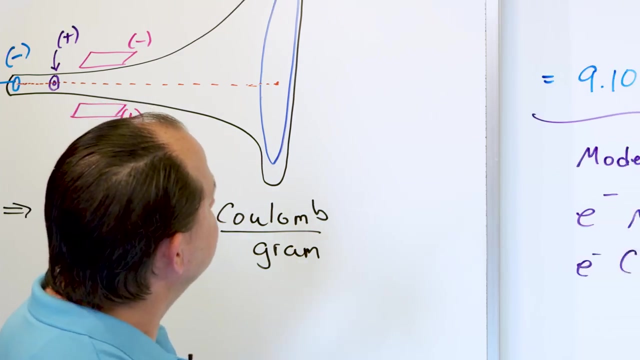 right is. the accepted value is 1.602.. One eight times 10 to the negative 19 coulombs. And so look at these numbers: 1.60218,, 10 to the minus 19.. And what did we calculate for that? It was just 1.602, 10 to the minus 19.. So that's. 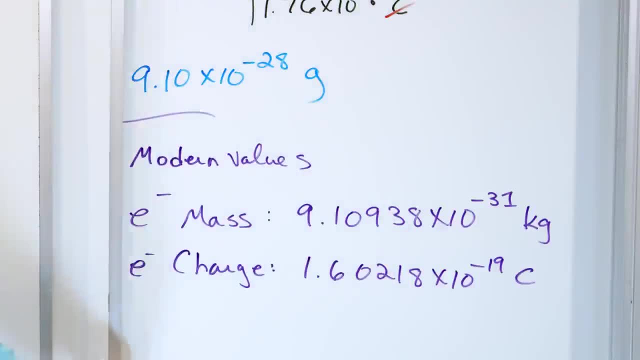 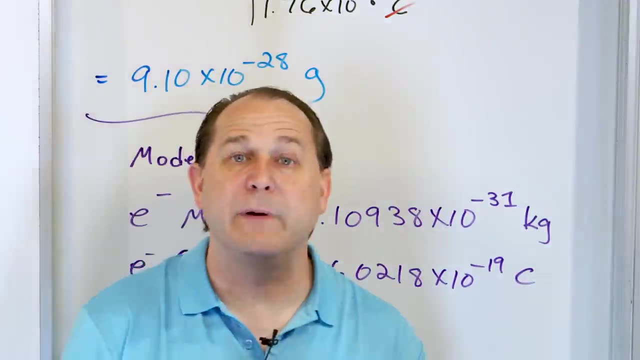 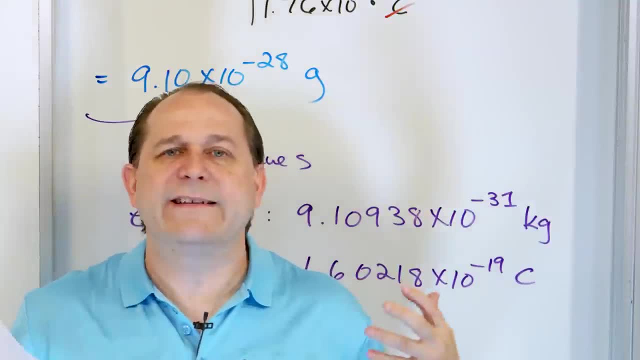 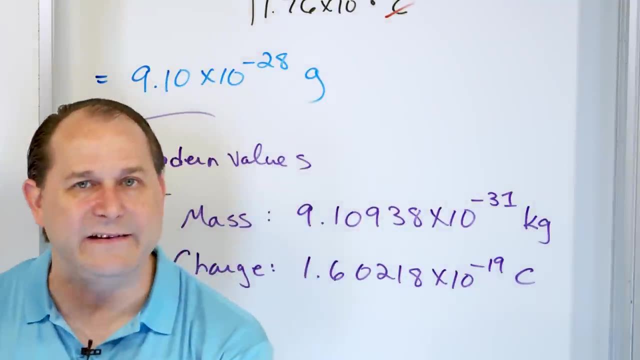 droplets of oil in a container. But just just take a step back, Okay, And realize that prior to the turn of the century, prior to the turn of the 1800s, into the 1900s, no one on the face of 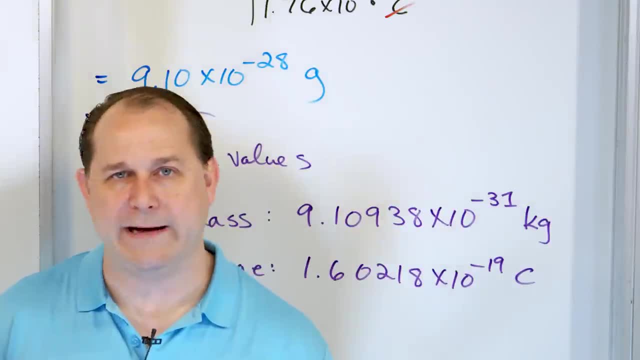 this planet knew that an electron was a thing. Nobody think about that for a minute. It's only been about. the year of this recording is 2022.. I hope people are watching it for many, many years in the future. So right now, as of the time of this recording, it's about 122 years. 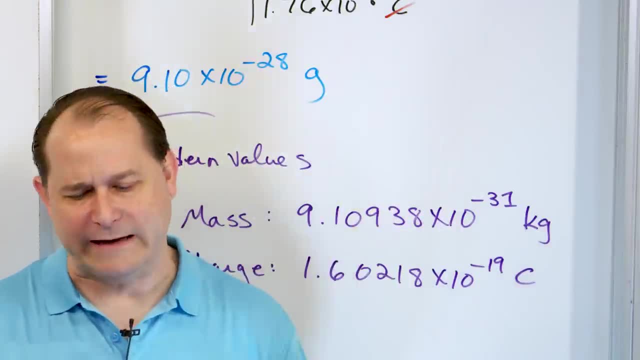 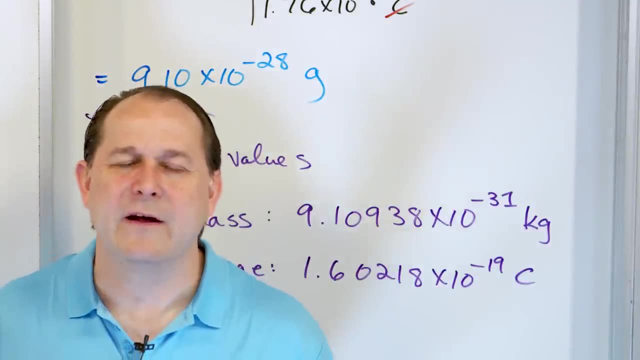 Since, and maybe even less than that, because this was discovered in like 19,. what did I say? 1909. Yeah, 1909.. Right, So about 120, 110 years, nobody knew when an electron was. 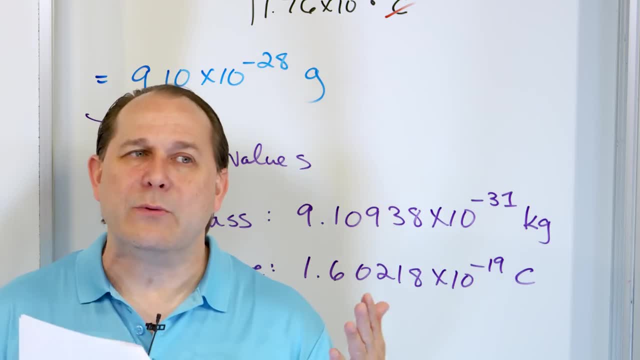 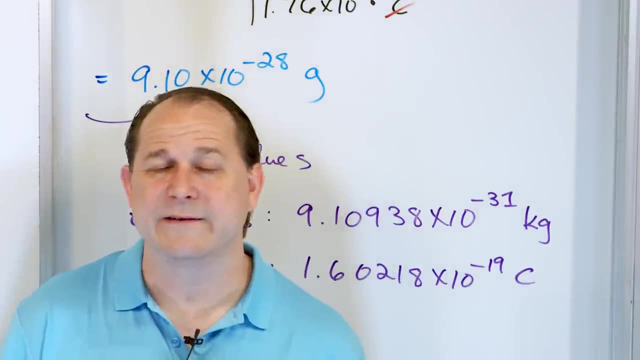 or that it even existed before this, these experiments. but we have gone from knowing now that electrons exist to- we'll talk in the next lesson- that protons and neutrons also exist, to knowing how chemistry exists, how to control chemistry to build things that can help our lives. and to enrich our lives. And so we've gone from knowing that electrons exist to knowing how chemistry exists, how to control chemistry, to build things that can help our lives, and to enrich our lives. and to enrich our lives, And so we've gone from knowing that protons and neutrons 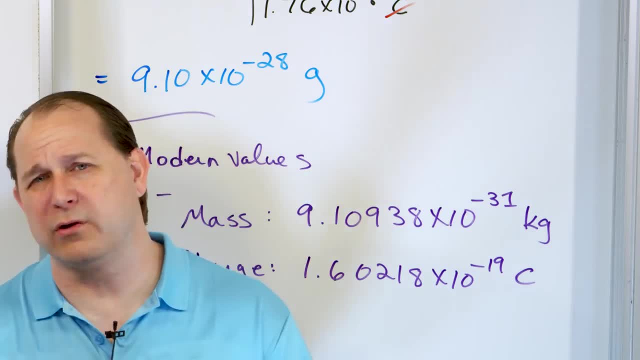 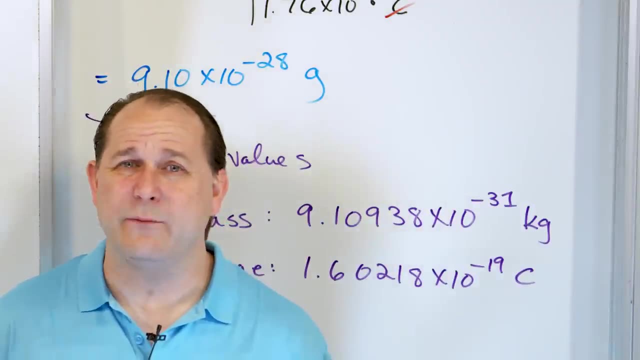 are civilization to making rocking engines and solar panels and computers and cell phones- all of that stuff happening in a span of about a hundred years. right, It's incredibly crazy that we were able to do this, that the, the collective minds of all these people have done this stuff. 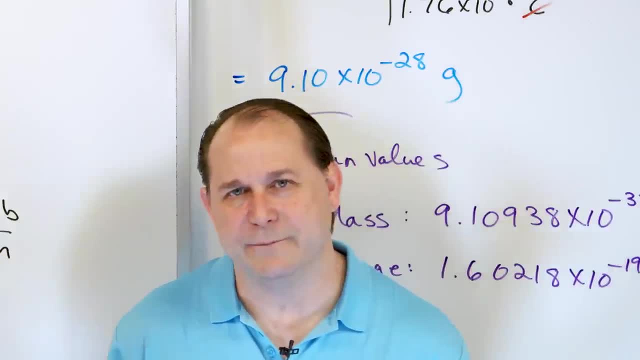 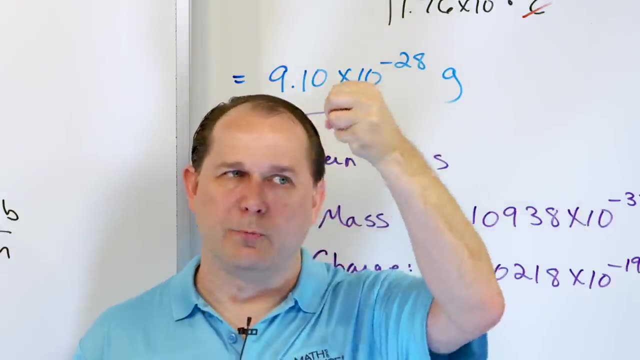 And here I am talking into a camera to pass this information to you, right? So this was a conceptual understanding of the discovery of the electron. It's helpful in the beginning to think of it as a little ball, Okay, So, yes, think about it, but in the back of your mind, just remember. 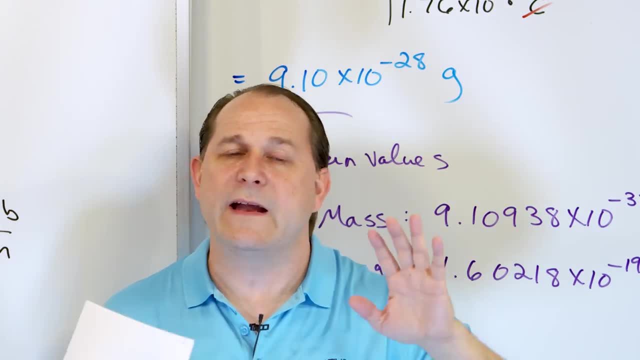 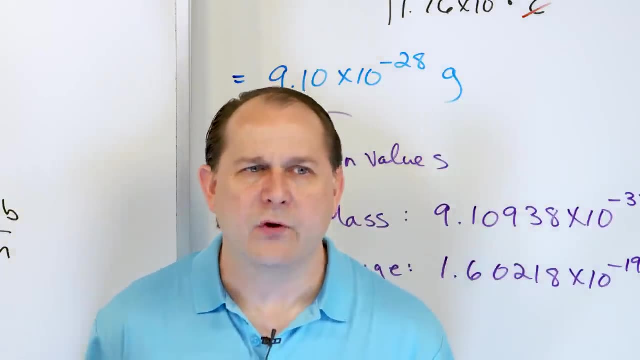 that there will come a time in the future when I tell you that that is wrong and that it's not a little ball. An electron is really a little wave. That is the punchline. It's a little wave. You have a bunch of questions now. What do you mean? a little wave? What's waving? Okay, What's what's? 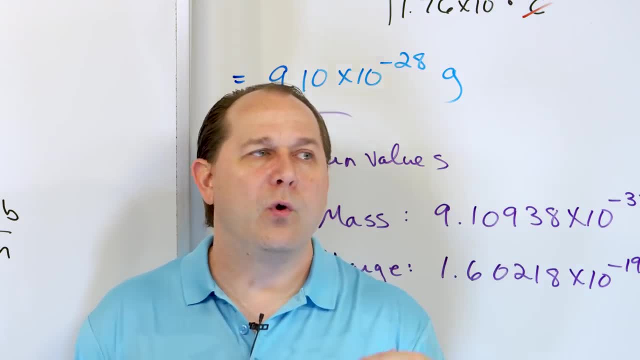 moving in water, water waves, the water moves right. For uh, for light waves we say electric and magnetic fields are waving. What's waving for an electron? Why is an electron made of a wave? Great questions. I hope you can figure out the answers, because we don't actually know the answers. 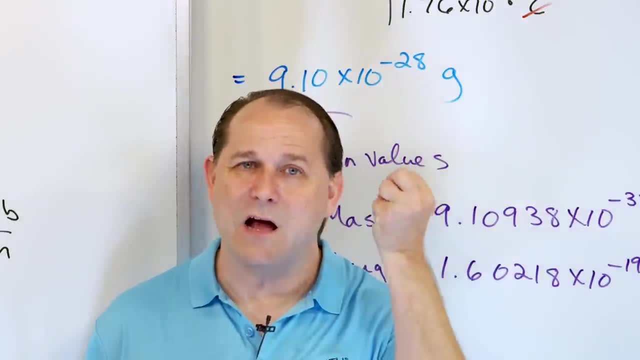 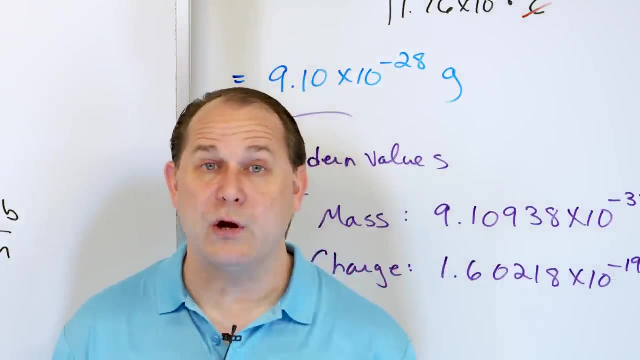 to a lot of these questions. but we know that an electron is not a little solid ball of like a bullet or something. It is a wave And I'll give you a little bit of a preview when we get down the road. uh, much more, much later when I do a a more of a lesson on introductory quantum. 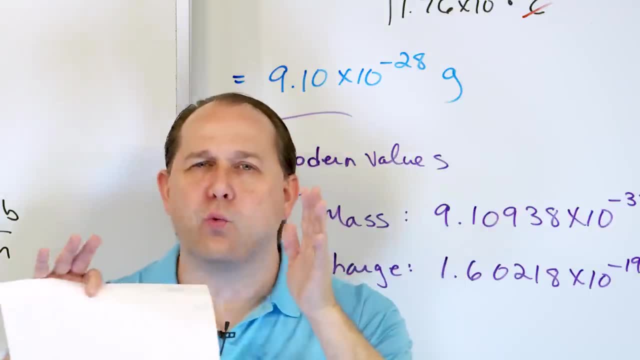 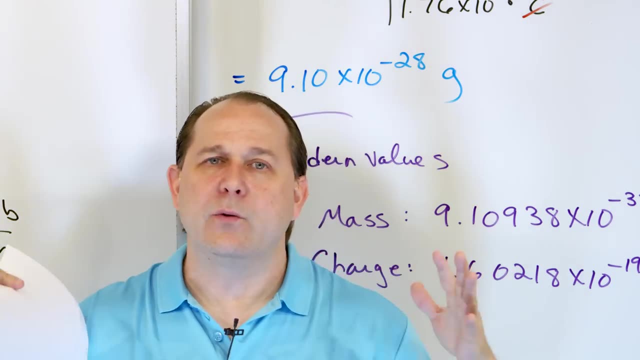 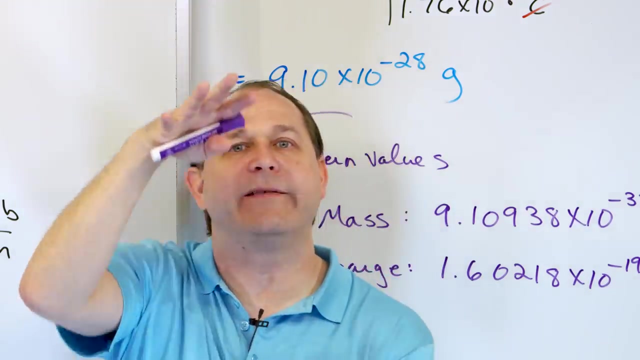 mechanics. Basically, when we, when we shoot waves, actual waves like either water waves or even light waves at slits, at two slits- the light waves and the water waves- they interfere with each other. That means the crest and the trough they line up and they either add to get bigger or they. 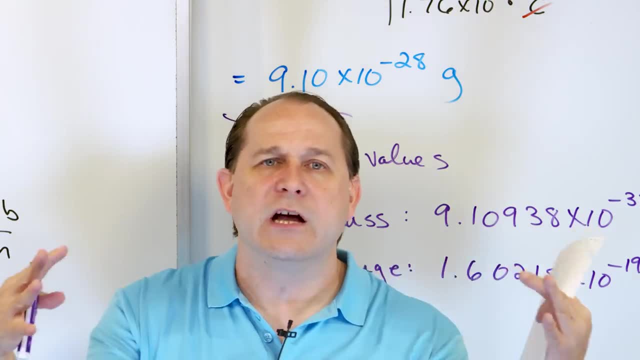 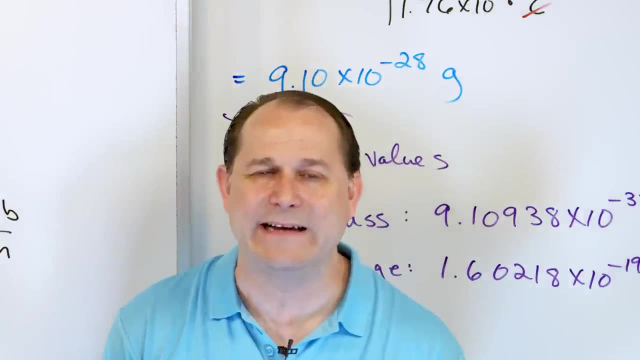 subtract to cancel each other out, because waves, when they collide like this, after they go through a pair of slits, they interfere and they add and subtract And we can see the interference. We know exactly how that happens. We have the all the math. We know how all of that happens, but it 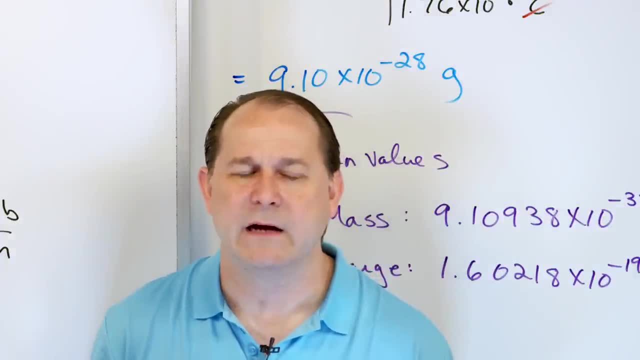 turns out, when you shoot electrons at a pair of slits like this, they don't behave like little bullets that just go through the slits. They actually interfere with each other And we see an interference pattern And we know exactly how that happens. And we know exactly how that happens. 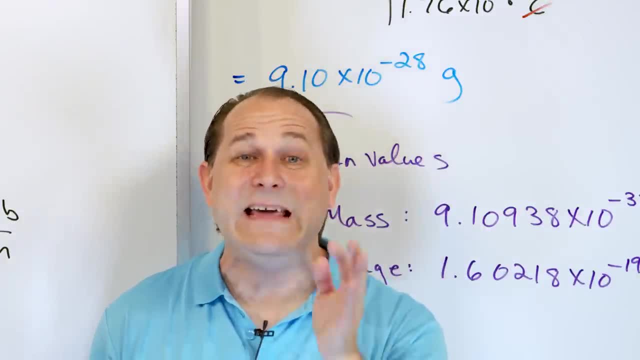 On the other side of the slits when we shoot electrons. even if we only shoot one electron, we still see an interference pattern on the other side. So we know that there's some kind of wave character to electrons And we know now from quantum mechanics that every piece of matter 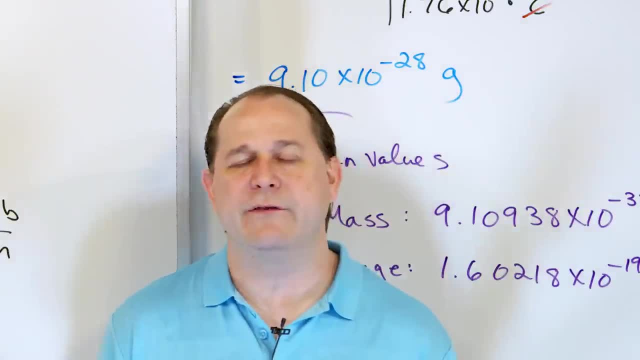 around you has some kind of wave character. Everything around you is basically made of waves. Now, what is waving? Why is it waving? How fast is it waving? Those are all things for a different lesson on a different day. Here we're just learning. how do we discover what? 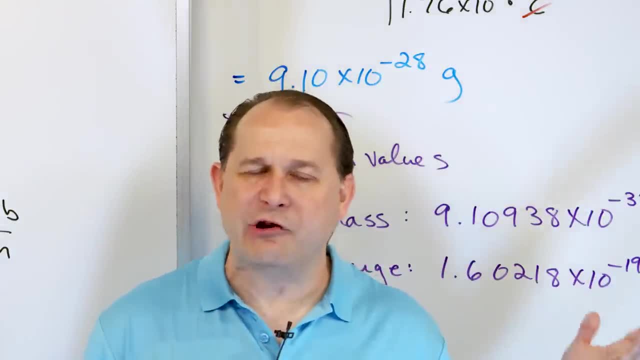 an electron was and how and what the charge and the mass of an electron is, And that we could use these experiments to get pretty close to modern day values. As we go through chemistry you're going to know and realize that everything chemically is happening because of electron. 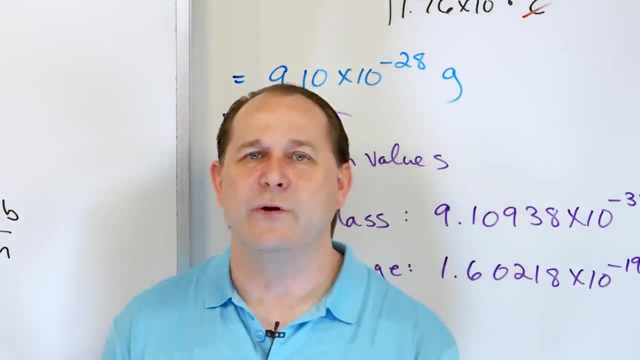 transfer or electron sharing, And then, when we get farther into it, of course, I'll drop a bomb on you and tell you that electron isn't a little ball at all. that's orbiting, It's a wave, And all of our modern theories support that with very, very accurate experiments. 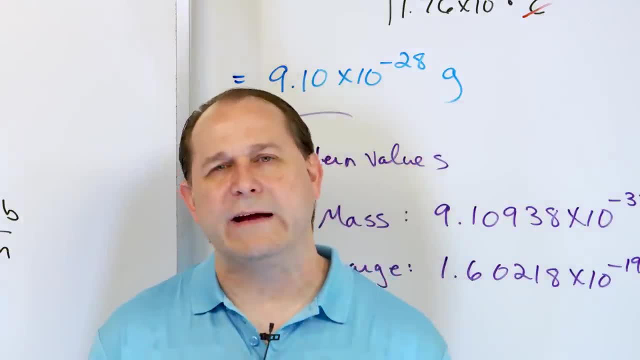 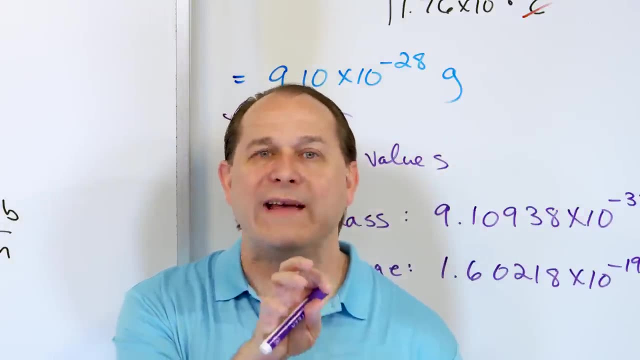 The best experiments we can do. So for now, watch this. Make sure you understand how we have discovered what the electron is. Follow me on to the next lesson. We'll talk about how the structure of the atom was actually deduced, And we'll learn about the protons and the neutrons, of course. which are in the center of the atom.